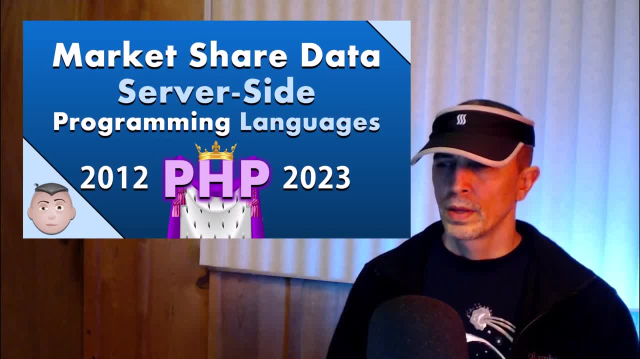 wrong about things near the end of this video And it's hard to debate that reality about humankind That the majority of us can be wrong. But before we get sidetracked too much, let's dig into some things that have a more solid foundation in objective reality. 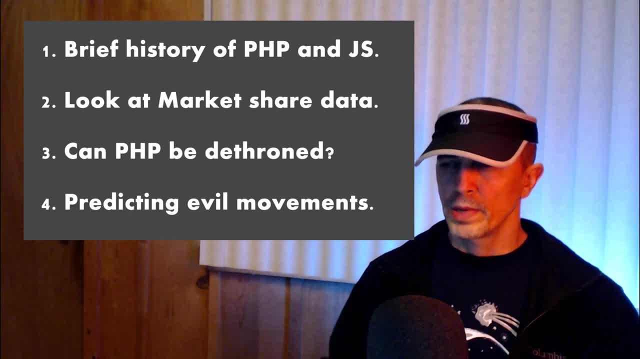 The first thing we'll do is discuss a very brief history of both PHP and JavaScript. Then we'll talk about how we can use it to create a more solid foundation in objective reality. Then we'll look at market share data for server-side programming languages in 2023.. 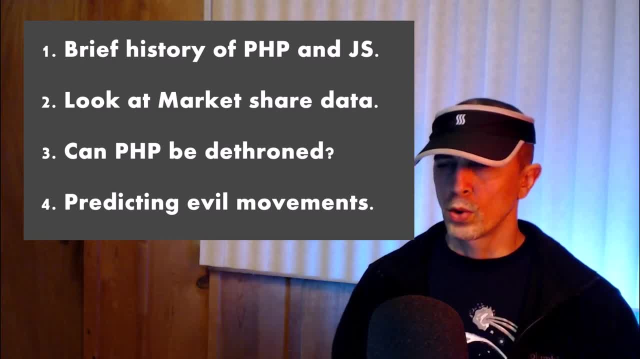 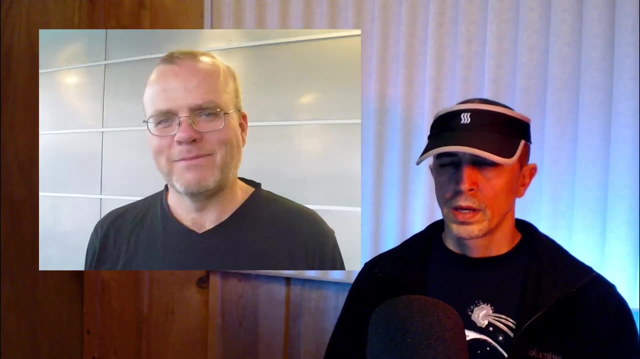 Then we'll discuss whether or not PHP can be dethroned And finally I'll make a prediction about greed-based movements and various entities that desire the death of PHP. So let's first start with a brief history of PHP. PHP was first conceived between the years of 1993 and 1995 by Rasmus Lerner. 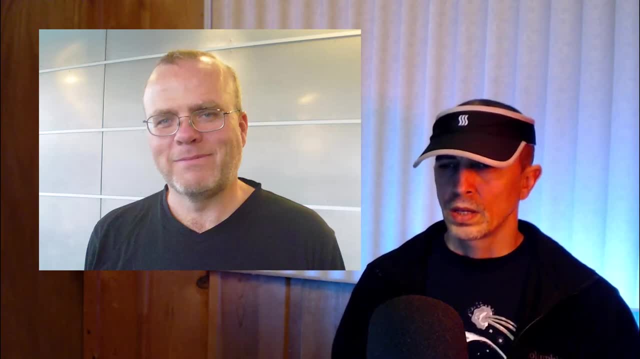 He wrote several CGI programs in C which he used to see who was looking at his online resume and to maintain his homepage. He then extended it to process forms and interact with his databases. It was created and conceived as a server-side backend programming tool for the web. 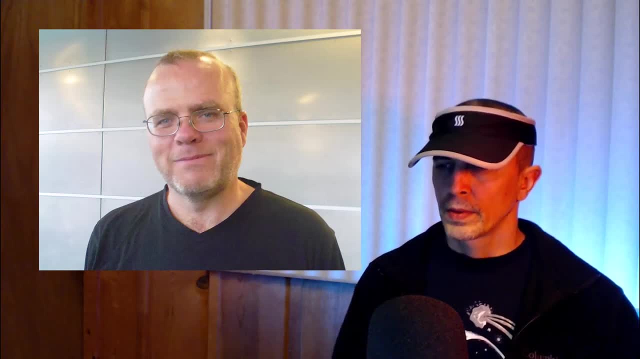 Its source code cannot be viewed like other technologies. It gained popularity over the years and has remained consistent as the top server-side development program for the web. It remains the clear favorite in 2023 according to market share data. Now a brief history of JavaScript. JavaScript was created by Brendan Eich in 1995 for the Netscape browser, which enjoyed dominance in the early Internet before Microsoft's Internet Explorer dethroned it. JavaScript has essentially always had server-side capabilities, but in early years it has been backfired. 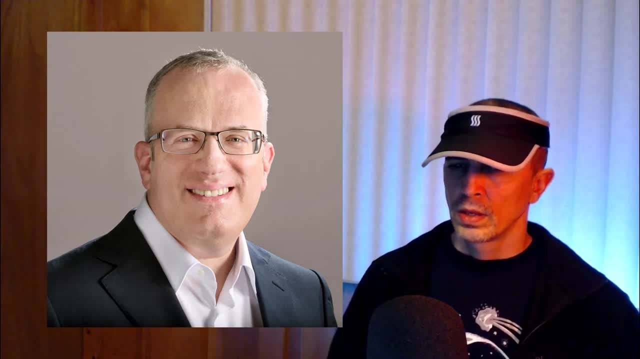 in early years. it has been backfired from its earliest days. even in the Netscape browser it had server-side capabilities, but JavaScript server-side programming never gained popularity for various reasons that we can discuss more in depth in future videos and you can let me know if you want to hear about. 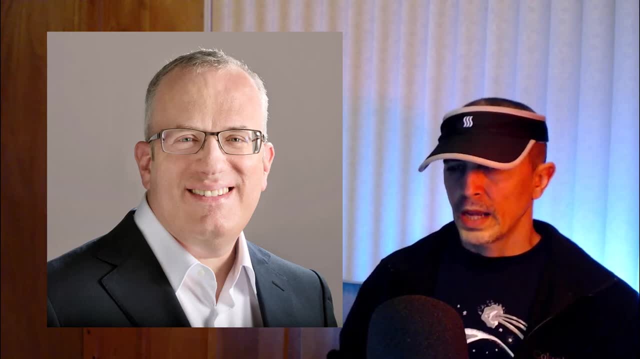 stuff like that in depth. when JavaScript then gained popularity as a client-side, front-end web development tool, because that was its primary conceptual function and its source code can be viewed by anyone- in order to hide or mask its source code, it would have to be obfuscated it. 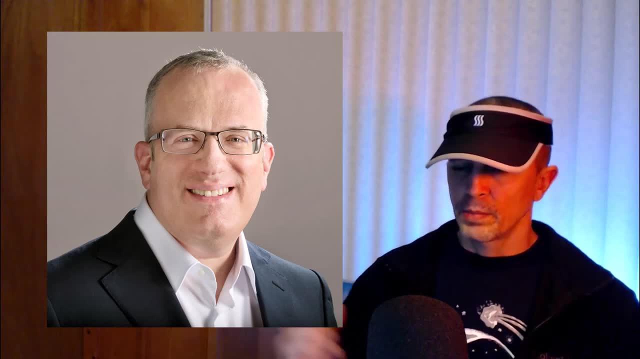 would have to pass information to something like PHP, which is not viewable source code, or you would have to obfuscate data in order to mask that data or, if you wanted to mask or hide your application's programming so it can send viewable data to the server-side development languages such as PHP and other. 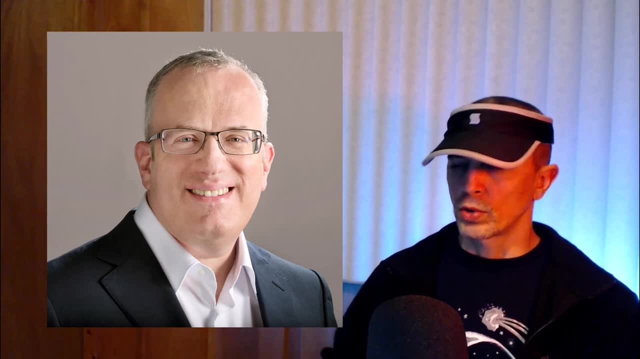 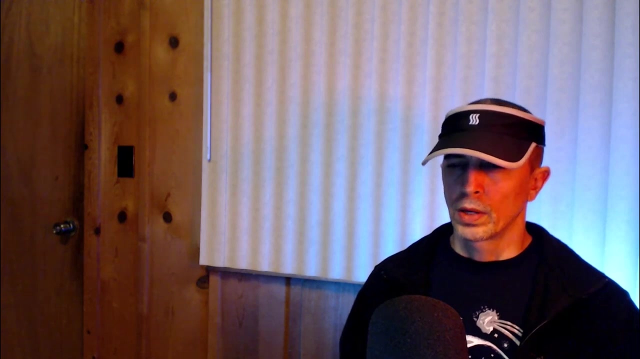 server-side programming languages whose source code is not viewable, which, at that point, what PHP does with it cannot be viewed. so the way that JavaScript handles data can be viewed by everyone, and the way that PHP handles data cannot be viewed by everyone. now my personal relationship with both. 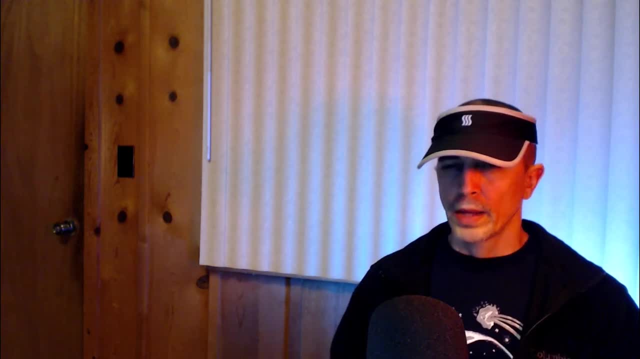 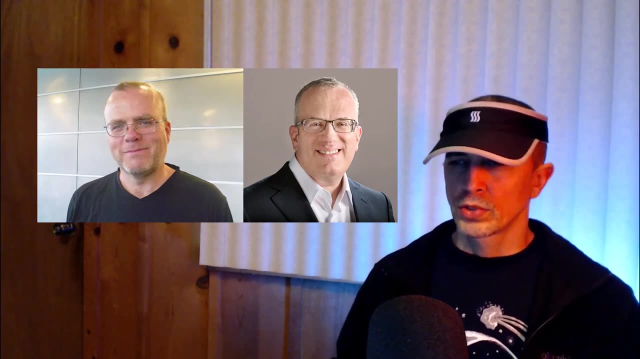 PHP and JavaScript is one of great respect for the fact that I have a lot of experience in the project and great admiration for both technologies and if one looks at my video numbers, they will see that I have way more JavaScript tutorials than I do for PHP and I want to see both technologies. enjoy a very long life and see both of them to continue evolving. I also use node. I use Python, Java, Etc where I believe they are best applied and most useful in my projects. so if my project has no need for node or no need for Python and PHP can handle it all very well and quickly and efficiently. I'm going to use PHP over node or Python, but there are certain instances where node or Python might be a better choice than PHP for just one or two things, but for the thousands of other things that PHP can do, PHP is the better choice, and node and Python cannot. 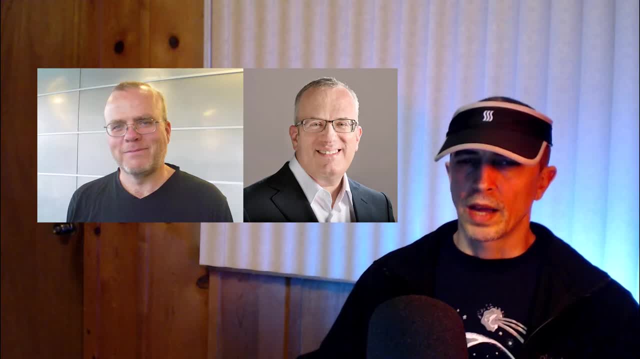 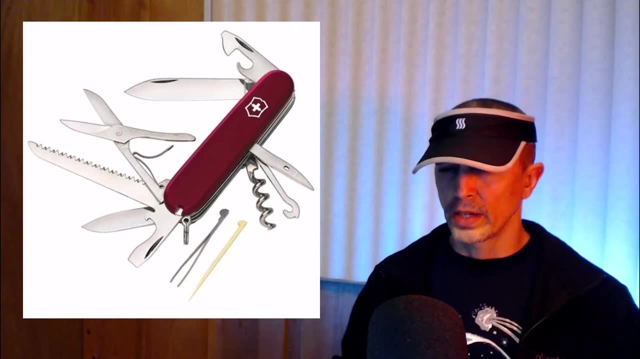 do all of those thousands of things that PHP can. now they all have their place, and I refer to PHP as the Swiss Army knife of server-side development, much the way I view JavaScript as being the Swiss army knife of client-side front-end development, so server-side being the back end and client side. 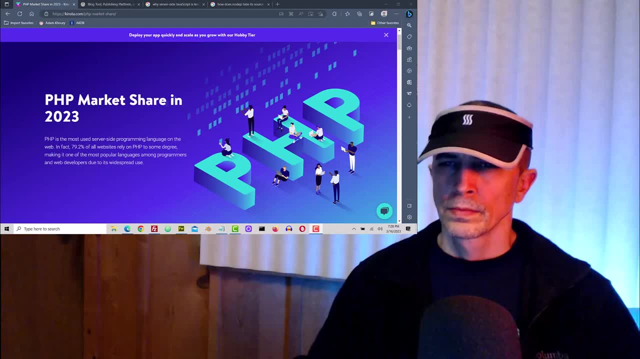 being the front end of development now, when you're researching the market share data for server side team software versus threadware, this is where our atra probably will benefit the most from the strategy we've taken now. so we're giving terms and conditions ofZY writebot code window to this. 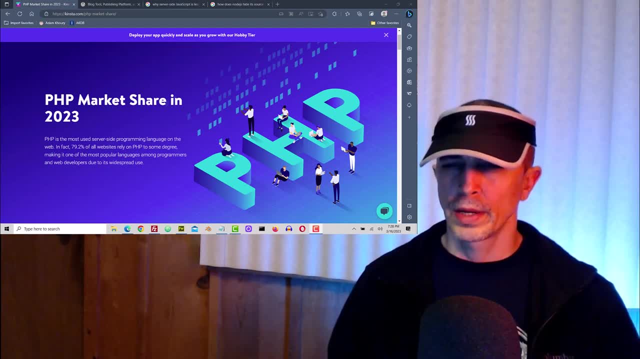 database, isicking the civ, a good opportunity for community writing's of the whole thing, and the 히r yo to6- one of the great prizes in this app page has- was inspired by javascript: job finding in the backend programming languages that are dominating the web, your search queries and search engines. 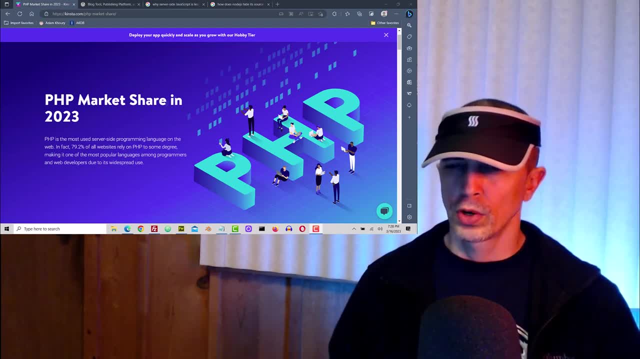 have to be correct. You know you can't just look for what's the most popular programming language in 2023, because that's not specific enough. We're talking about backend server-side development in specific, And you can't just go to some blogger's site or one of the entities that. 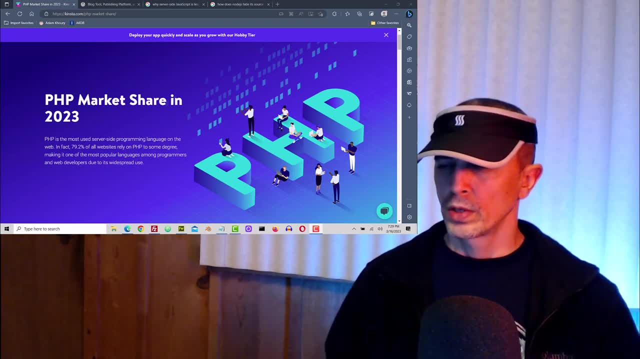 might have some kind of favoritism for one framework or another. You have to try to find entities that are known for dealing with data and statistics, or somebody that might be a little bit more objective without anything to gain by promoting one or the other. So I found a few. 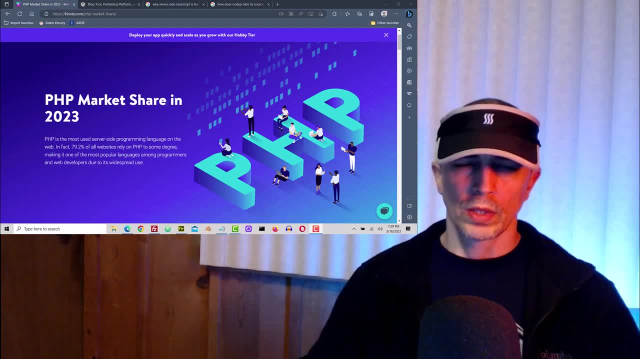 very reputable entities and we can take a look at what they say. And I also chatted with the chat GPT- artificial intelligence that everybody's going so wild about lately- And I'm going to show you a clip from that: what it had to say about PHP versus things like Node. 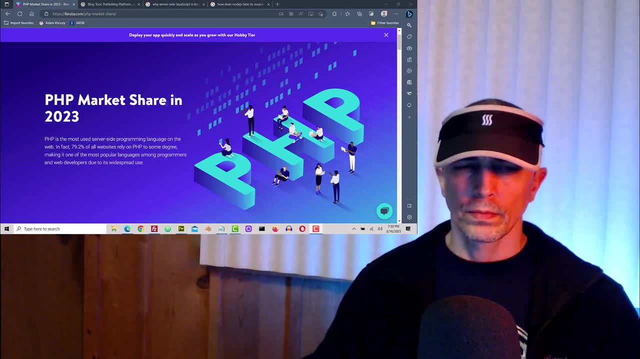 and JavaScript backend programming for the server-side. So here at Kinsta it says PHP market share in 2023.. PHP is the most used server-side programming language on the web. In fact, 79.2% of all websites rely on PHP to some degree, making it one of the most popular. 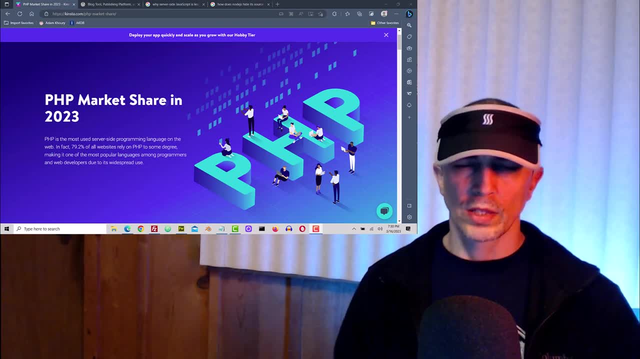 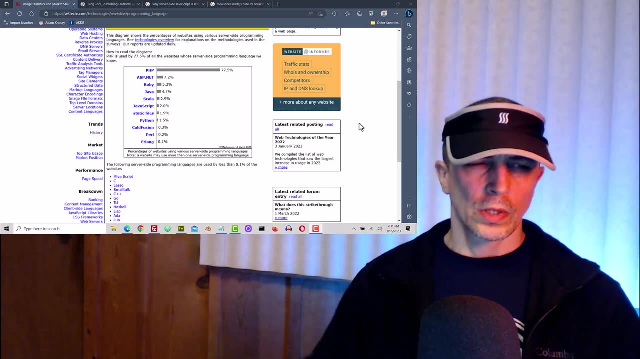 languages among programmers and web developers due to its popularity, And PHP is used by a large number of people and it's widespread use, So people who say that PHP is dead or dying are just wrong. Now let's take a look at w3techscom, which does a lot of data analysis and market share analysis. 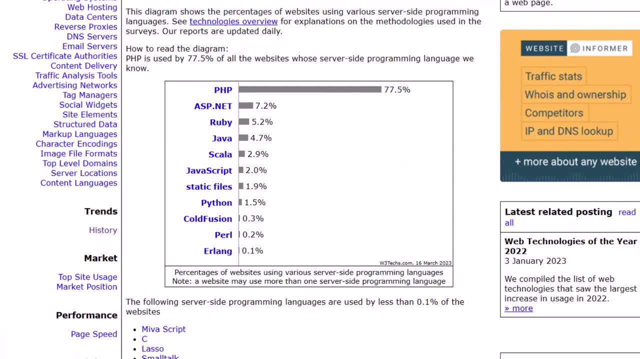 So it shows that PHP is used by 77.5%, where ASPNET is 7.2%. Ruby is 5.2%. Java is 4.7%. Scala is 2.9% and Java is 4.7%. Scala is 2.9% and Ruby is 4.9%. Scala is 2.9% and Ruby is 5.9%. Scala is 2.9% and Ruby is 5.9%. 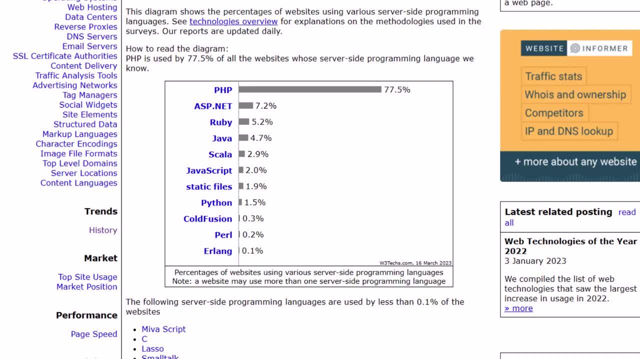 And, as I said, JavaScript is 2.9%…. JavaScript is 2%… And that includes Node and other libraries that are not Node, that are used for back-end server-side development. As I said, JavaScript has had server-side back-end programming capabilities since its. 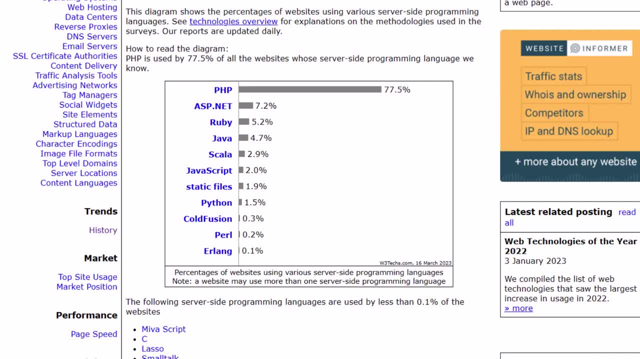 conception in the 1990s. So 2% here in this chart represents Node and every other JavaScript library or framework used for server-side back-end programming and we have static files at 1.9 percent, python at 1.5 percent, cold fusion at 0.3 percent, which cold fusion used to be a lot more popular, and asp. 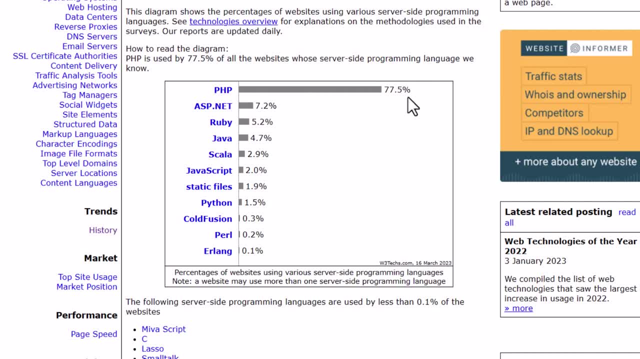 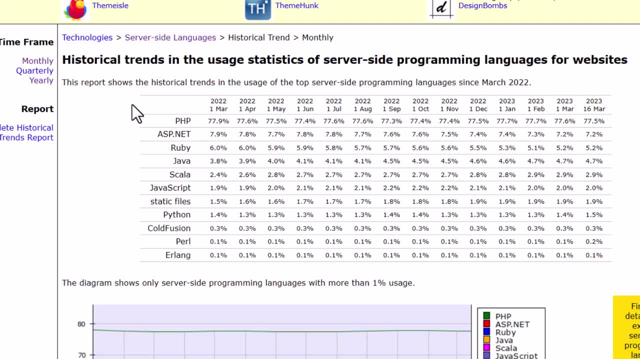 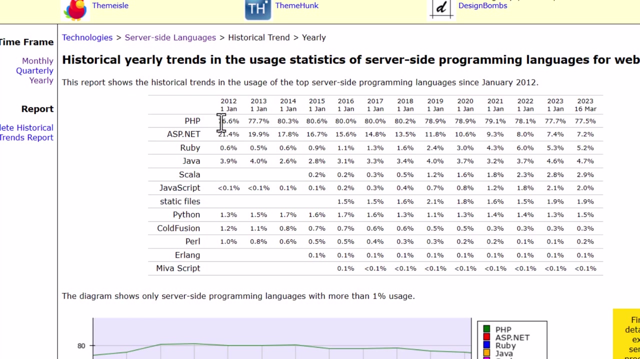 net used to be a lot more popular, but php has been consistent throughout the years and if you click history, you'll see a chart that shows from 2000. well, this is a quarterly chart, but let's go to yearly over here, and this is from 2012 to 2023. 2012, php was at 76.6 percent of the market share. 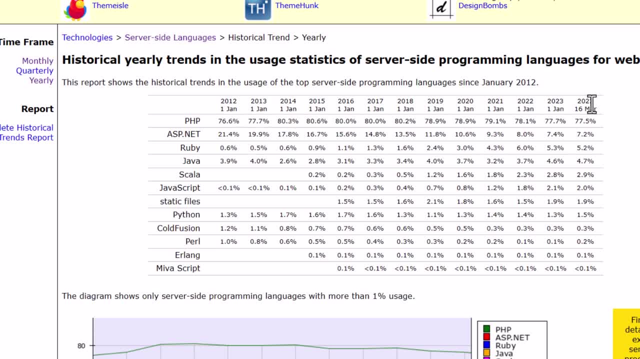 and it's remained consistent pretty much all the way to march 16- 2023, at 77, 0.5 percent. now look at aspnet: it's gone from 21.4 percent, consistently downhill, which, aspnet is microsoft's technology for server-side programming, so started in 2012 at 21.4 percent. 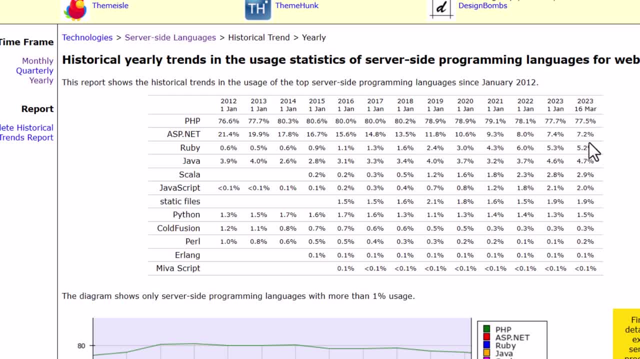 and it's now at 2023 at 7.2 percent. so it's gone consistently downhill. ruby has gone uphill. java has gone uphill slightly. java started at 3.9 percent 2012 and is now at 4.7 percent. scala has went uphill slightly. 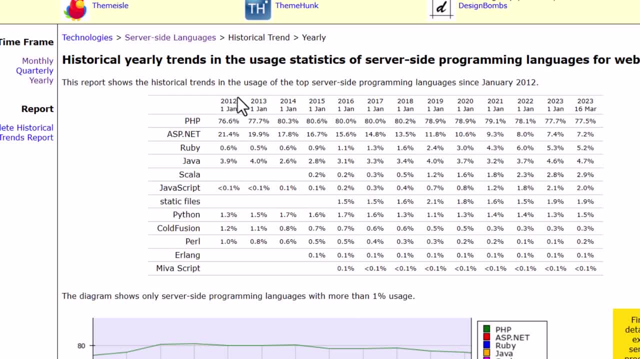 now. javascript was less than 0.1 percent in 2012 and now sits at two percent, and that includes node and all the other libraries for server-side programming using javascript or server-side communication using javascript. now we're going to take a look at javascript. 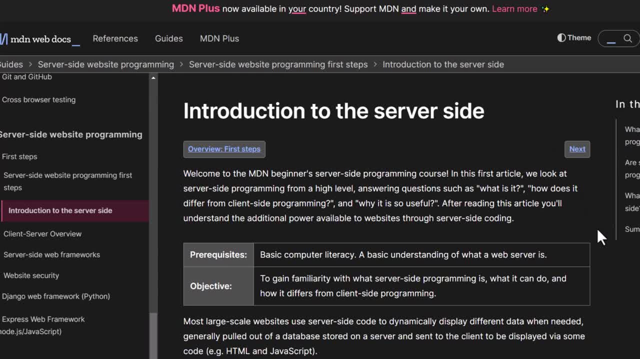 so that you guys can understand more about javascript if you guys had a limited access. just one more entity. this is a very reputable entity and honestly they're more javascript focused. they have more to gain by promoting javascript at mozilla foundation. then they do have promoting php and other things. they stand to gain more if javascript gets more popular. and let's see what. 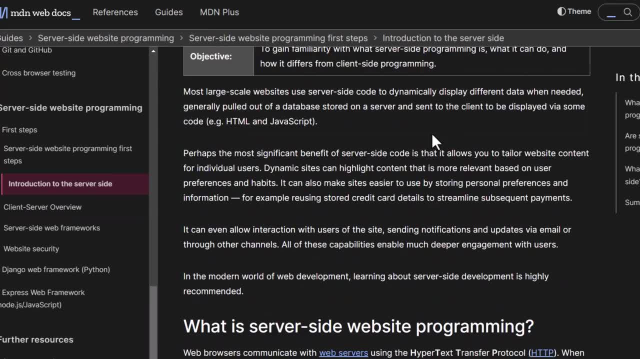 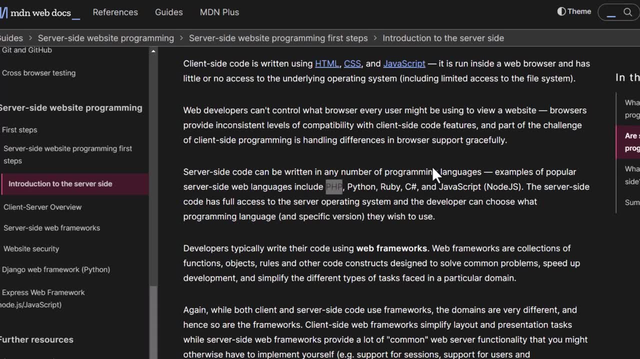 they say in their introduction to the server side. on their website little bit, we can read that server-side code can be written in any number of programming languages. example of popular server-side web languages include php, python, ruby, c, sharp and javascript. so you can see, even mozilla puts php at the front of the list for a very specific reason. 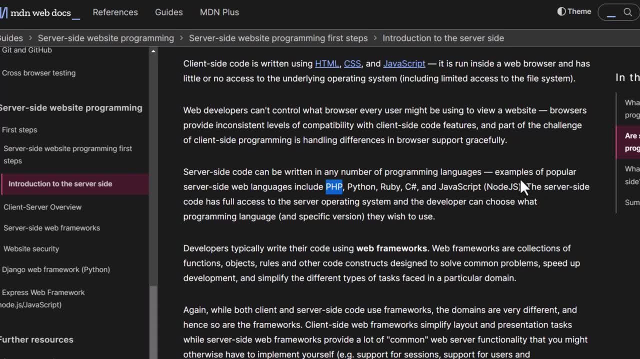 it's because php has the dominant share of the market in 2023. in years past and upcoming years, it will still enjoy that dominance in the market share. now something should be said about nodejs and python- server-side programming for the web. there's only a few things that that can do. 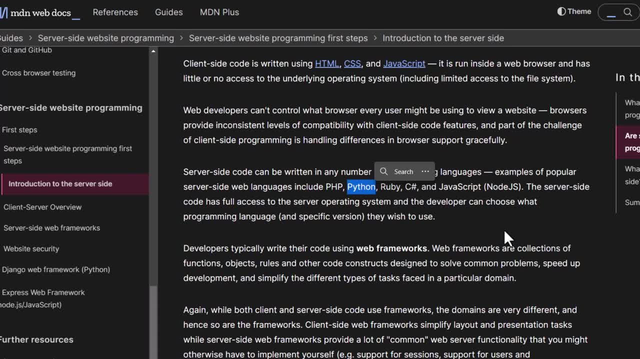 better than php can there's? i've worked with all of these technologies and there's only a couple of things that can do better than php. can that node or python can do better than php, but there's thousands of things that php can do that those other things can't do or can't do as well as php can't do it as efficiently, can't do. 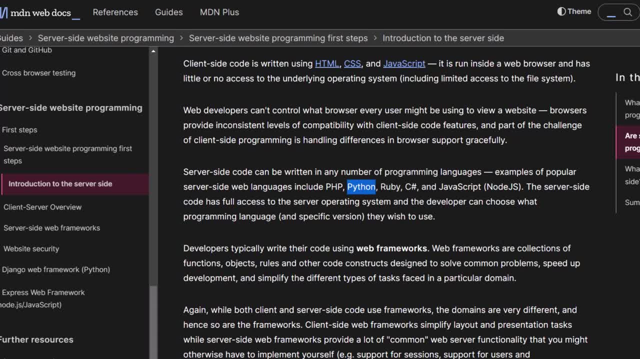 it as easily either, and php is just a more trusted technology for doing all of these things. like i mentioned, the swiss army knife of server-side development, php is just more trusted by more developers than on the web and php is just the most trusted überhaupt in terms of properties. 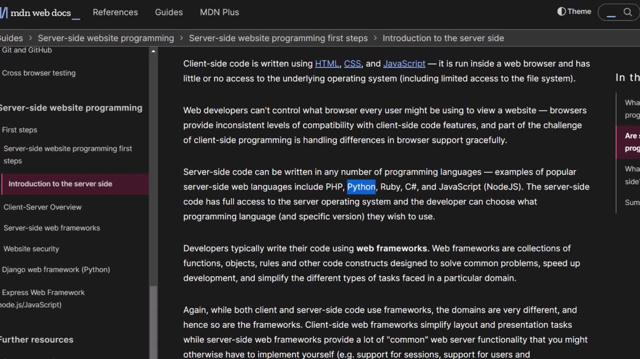 vine and windows, and why not get unaffected by php subscribers? but- and in this case, with a drama between unsonymous being 1983, rjk and more corporations and companies, and I don't care what any company says or any favoritism they want to show every large corporation if they know what they're doing with web development. 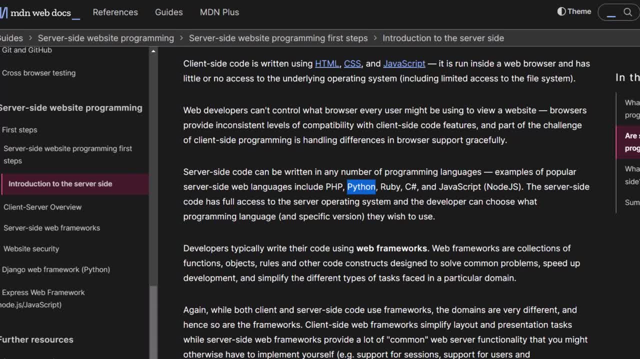 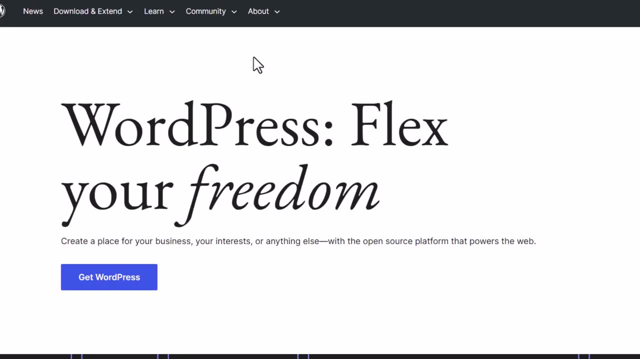 they're using PHP in their back end, And some might claim that, oh no, we only use Java or we only use Python. Well then, you're not doing much back there. Even Java on the back end, it can't hang with PHP. Now let's visit WordPressorg Now. you have to be careful here. 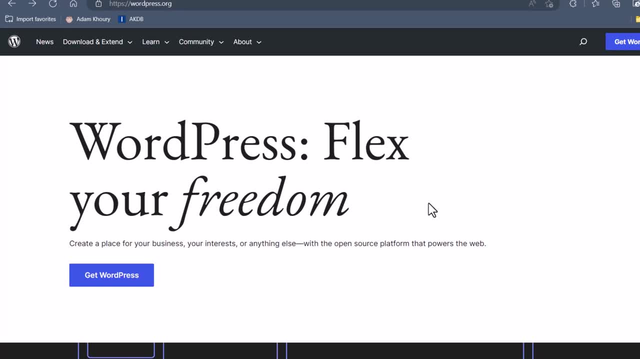 because WordPressorg is the official site for the free, open source WordPress software that people use for building their websites. Now, WordPresscom is a for-profit, paid service that is powered by WordPress software, but it is not the WordPress organization. It's not the WordPress software. 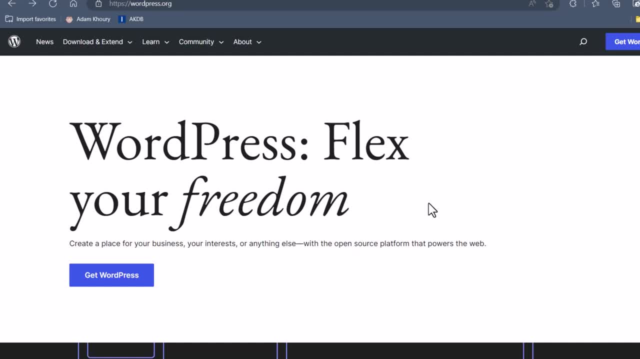 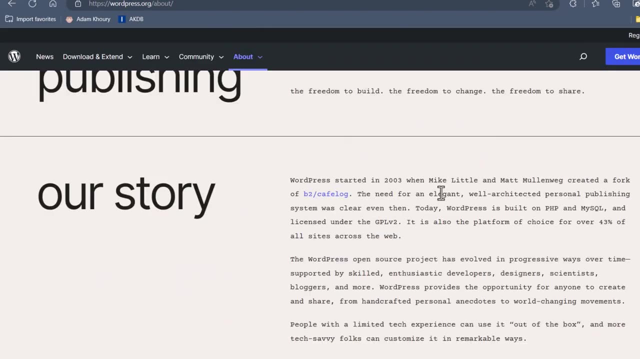 So If you go to WordPresscom, you're not going to get accurate information about what WordPress the software is, or what it's becoming and all of these things, So let's click on WordPressorg About. About WordPress. WordPress started in 2003 when Mike Little and Matt Mullenweg created a fork of the B2 slash Cafe log. 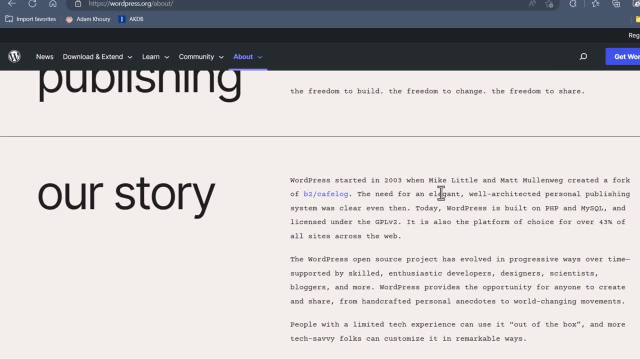 The need for an elegant, well-architected personal publishing system was clear even then. Today, WordPress is built on PHP and MySQL database and can also be used with MariaDB, and it's licensed under the GPLv2.. It is also the platform of choice for over 43% of all sites across the web. 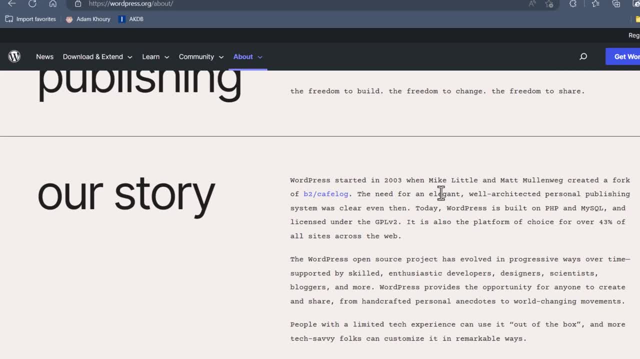 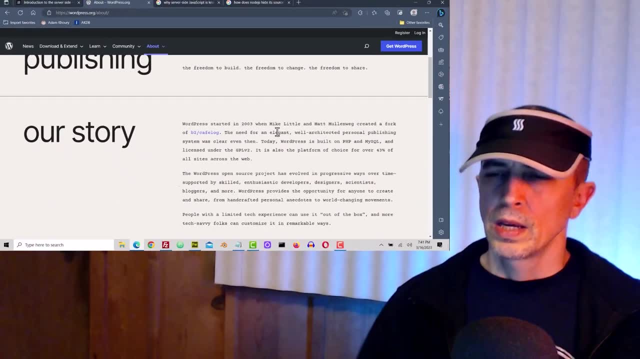 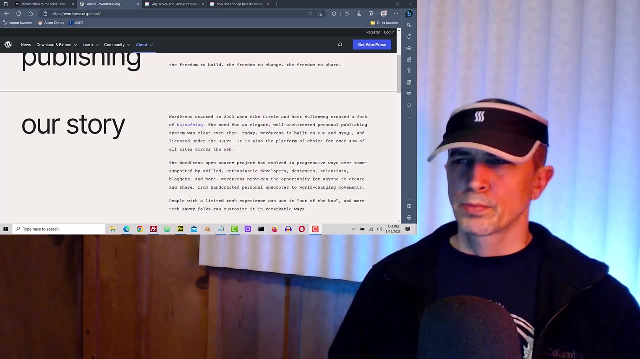 So 43% of every website on earth is powered by WordPress, which itself is powered by PHP and MySQL. Now you might think to yourself: well, wait a minute. PHP is probably only so popular because WordPress is using PHP, So that's why it has such good market share numbers. 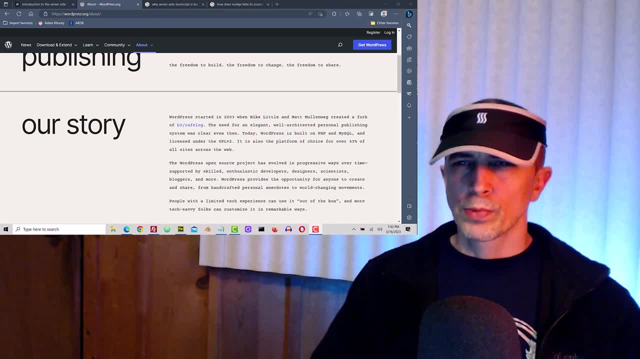 And I think that's wrong thinking because WordPress. I think it's the other way around. I think WordPress is so handy and useful and used by so many people because it's using PHP and not the other way around. But PHP isn't king because of WordPress. 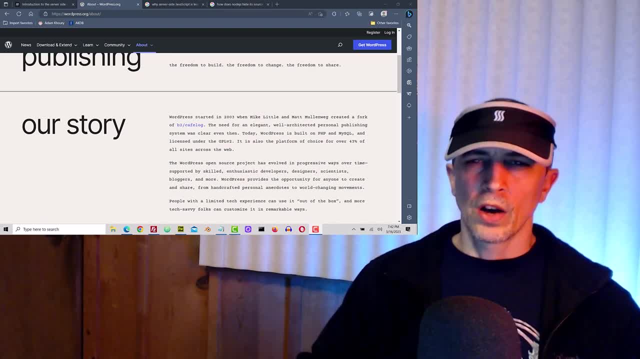 WordPress has become king of CMS content management systems because it uses PHP and MySQL. That's what I believe the reality is, And we can debate that. but it's clear to see that even if you killed WordPress, tomorrow another tool would have to come up in its place. 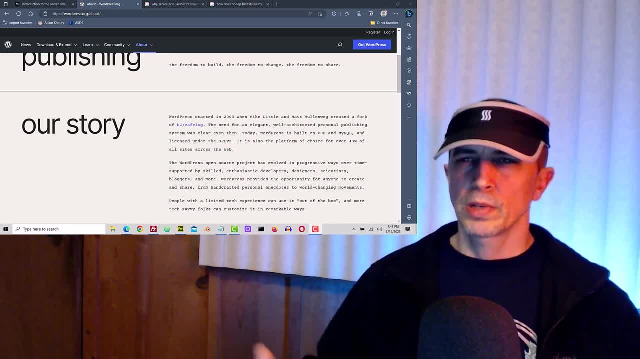 Another content management system would have to come up in its place to become popular. Right, WordPress is, and it would have to use something like PHP to be as useful, handy and easy to use and so have such a wide array of features and functionality. because it's using PHP, not the other way around. 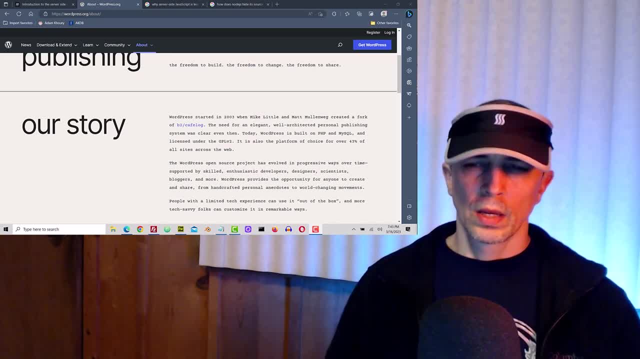 And even if you remove the 43%, that still leaves PHP as the dominant server-side programming language. Even if you remove that 43% Of all sites using WordPress, PHP still dominates all the other server-side technologies. But, like I said, WordPress, I think, is only so popular because it uses PHP. 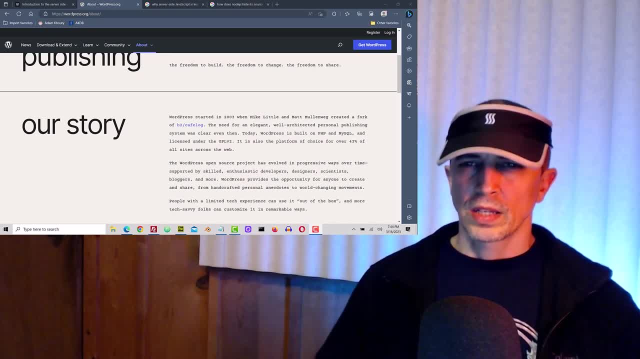 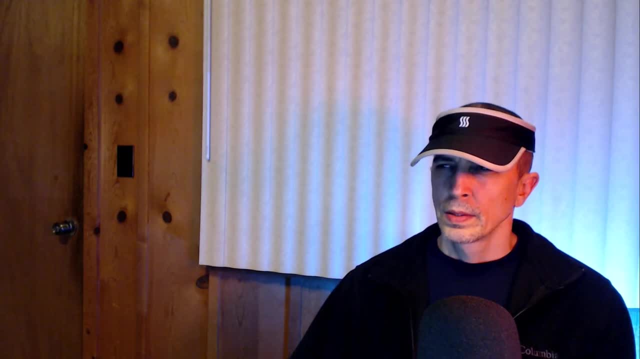 And, like I said, another tool that comes up to take its place is going to have to use something like PHP if it wants to compete with WordPress. I want to quickly mention that there are lots of entities that you can get Good market share analysis data from that are not biased, that are not just fly-by-night bloggers and that have no special interest in siding with either Node or Python or PHP and things like that. 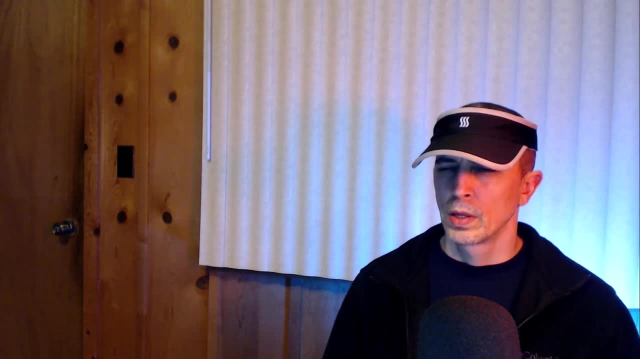 There's plenty of good sources to get the market share data from, And I even saw the market share data from Forbes, the business analysis entity. Even Forbes understands that PHP holds a large share of the market- The largest share of the market- consistently over many years and even today, in 2023.. 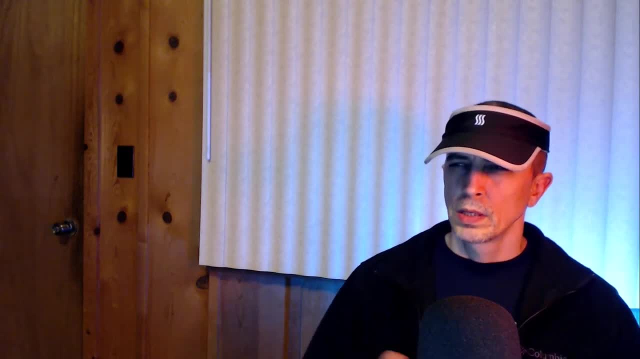 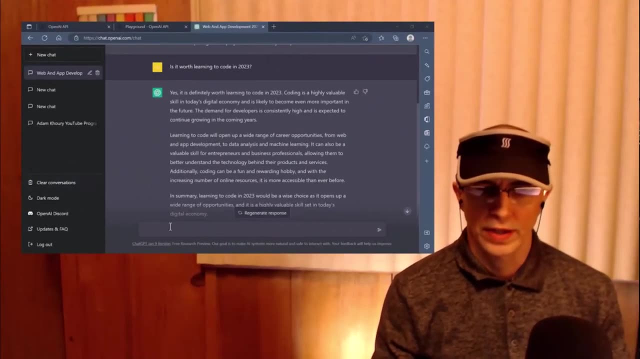 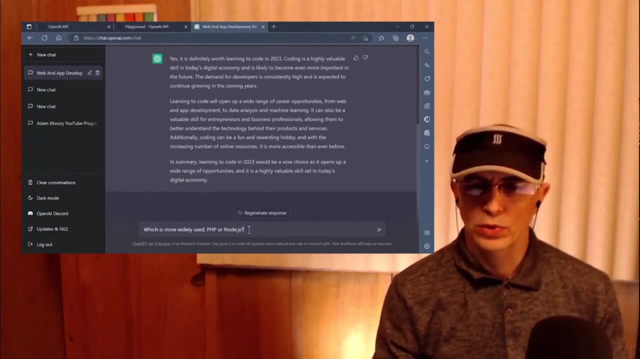 Now I'm going to quickly play the clip of me chatting with ChatGPT And see what ChatGPT has to say on the matter. Okay, Now let's get controversial here. Which is more widely used- PHP or Nodejs? 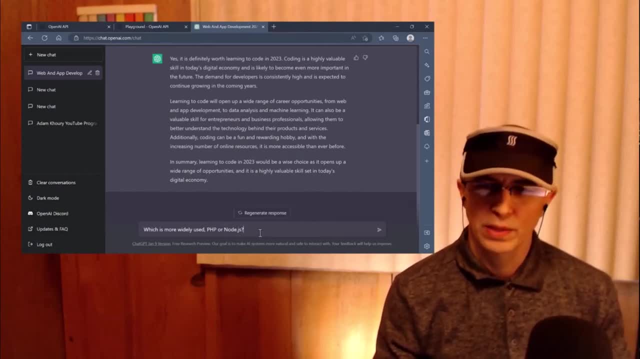 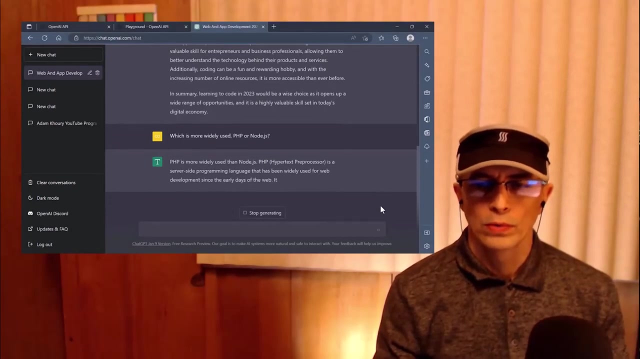 And I'm asking you this because I hear a lot of people saying that PHP is dead and that Nodejs everybody's using it. nobody's using PHP anymore And I just wanted to dispel that Uh-oh. A lot of people are not going to like this answer. PHP is more widely used than Nodejs. PHP Hypertext Preprocessor is a server-side programming language that has been widely used for web development since the early days of the web. It is particularly well-suited for building dynamic websites and is the language behind many popular content management systems like WordPress, Drupal and Joomla. As of 2021, PHP is used by about 79% of all web browsers. Nodejs is a relatively newer technology, which is a JavaScript runtime built on Chrome's V8 JavaScript engine. As of 2021, Nodejs is used by about 2% of all web browsers. 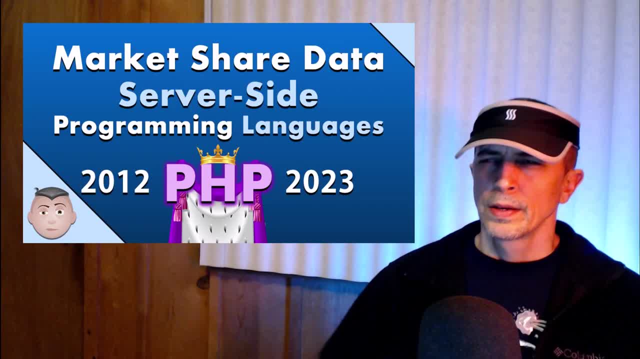 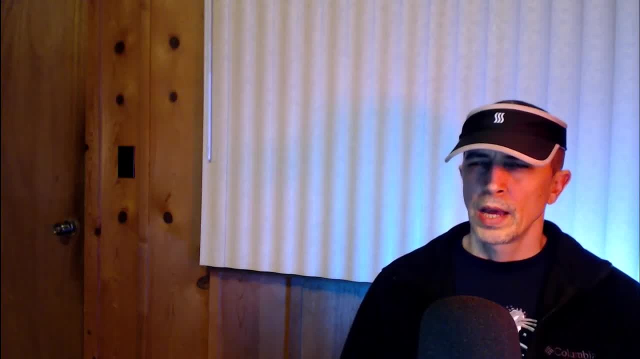 Nodejs is a relatively newer technology, which is a JavaScript runtime built on Chrome's V8 JavaScript engine. All right, Now let's quickly discuss whether or not PHP can be dethroned, when it will be dethroned and by what. 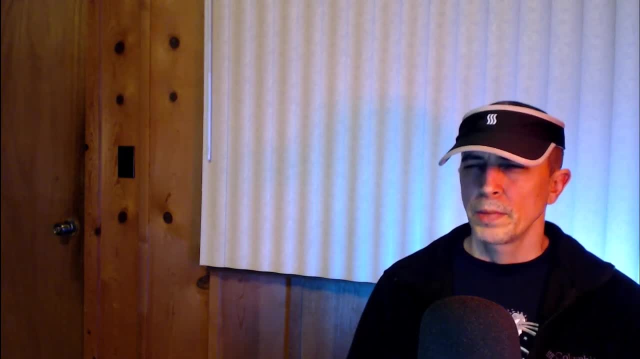 Of course PHP can be dethroned, But if it gets dethroned, I believe it's going to happen in the face of lies, misconceptions and favoritism by big tech that has vested interests in making other technologies come to the surface and have a higher percentage of the market share. Because there are a lot of big tech entities such as Google, Facebook and other entities like Apple and others, And it will easilyunku all companies that have invested a management interest in making other tools and frameworks that they may have developed or work on their own on top of interests that start with some new engines. 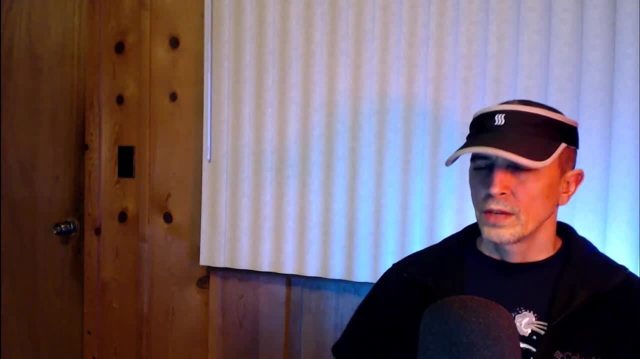 Let's get theität put together. It might happen to PHP that's being used. I just think is Est attractive because it's actually straightforward. Next slide: Let's get the dass t. oh, the hit tile again. Let's get that. Let's see. 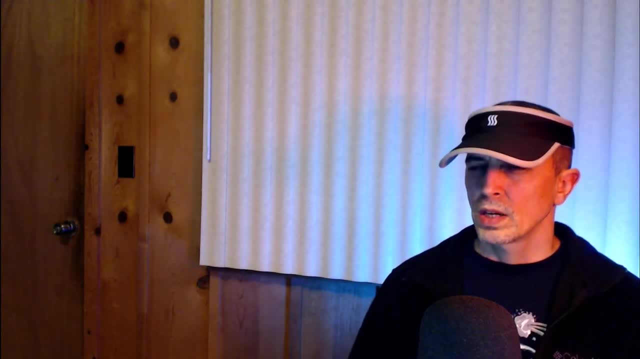 Let bet something in there. Let's get it. It's all right, It's going to happen. It's going to happen, brainwashing. but even if that's not the case- and it's not evil greed agenda behind the death of php- all things change. nothing stays the same forever. something will eventually come along. 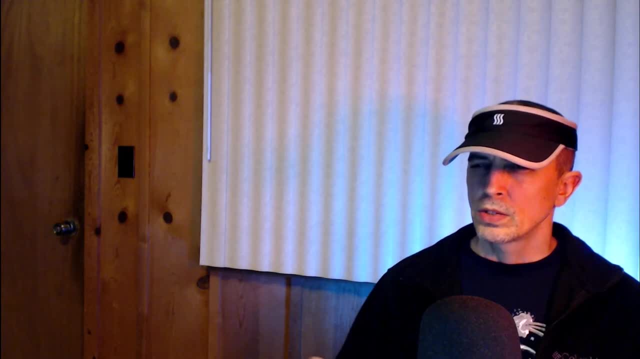 that has maybe better ease of use, better speed, better functionality than php. so you can't really say that php is just going to be around forever, and of course things evolve and things change, but when that happens nobody knows. but for sure in 2023 and the next coming up few years. 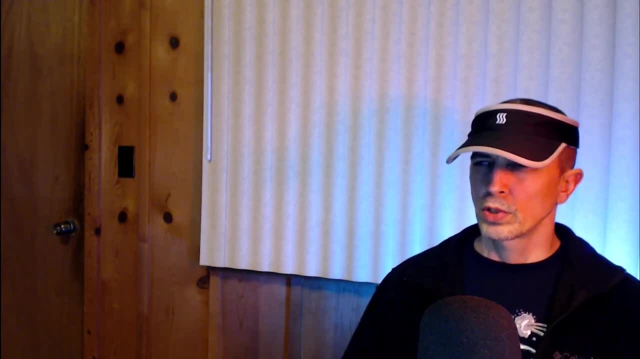 till 2027. i believe php is going to enjoy a large, healthy share of the market the way it has for the past 10, 15 years. it's not going to be so quick and there's a lot of people that will today say: actually for years, for the last five years, they've been saying php is dead. php is dying and 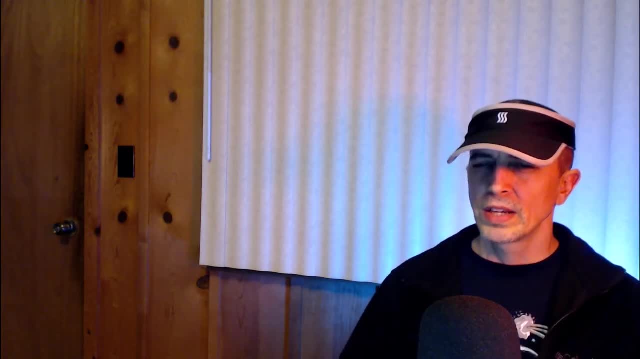 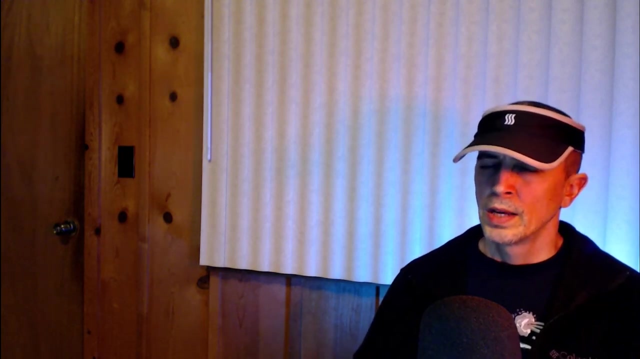 these people are completely bonkers. they're living in some kind of fantasy land that is so detached from reality it's hard to even explain how cuckoo bananas these people are. now that leads us into the topic of me predicting evil movements. i'm going to predict that there are going to be a lot. 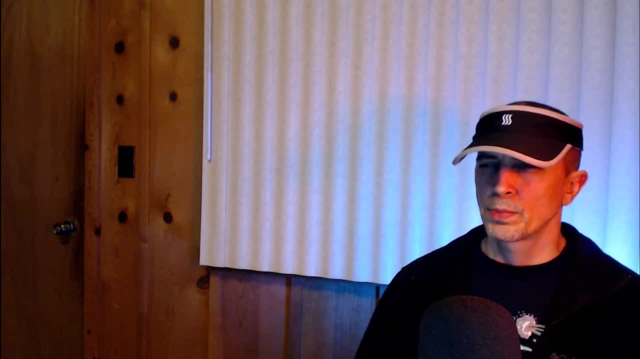 of evil movements coming against me, against php, and you can already see that has happened over the last five or ten years- because php is king and when you're the king, everybody is going to be trying to stab you in the back, to take what you have or to take the power and control that you have, and it's not like php is. 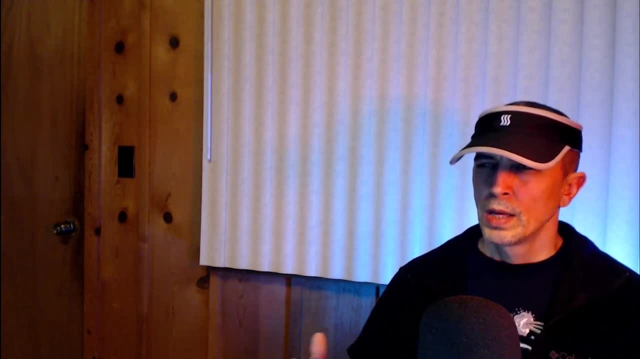 even profiting much, the, the whole management team and the whole organization. that is php. it's a free and open source programming technology and it's going to be a lot of fun and it's going to help everybody who wants to keep up with their life. so if you have blown out of the Buddha and 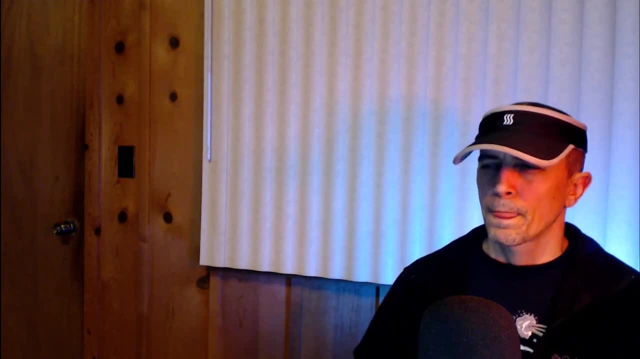 you think i'll totally and blow you out of the celiac. you'll deep black out. if i don't tell you everything that it is, that end is really gonna fall off the grid. whatever you're dealing with is going to happen now. php will not continue to come in. this adalah: 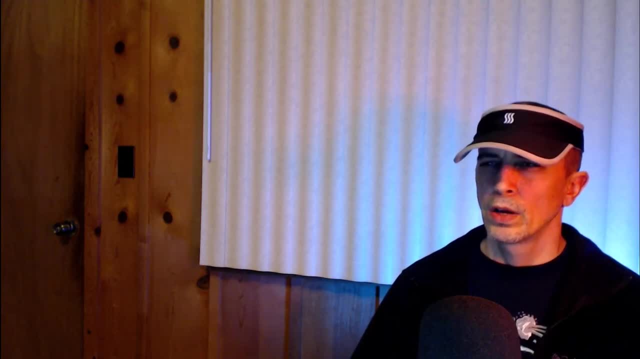 it is an until this point to do and go to doesn't mean it's fucking hands off. this long term, 50 to 60 minutes School year and history is going to hold the którelen and with your schedules and so on, and they're not going to have much money. representatives, how far well did a big 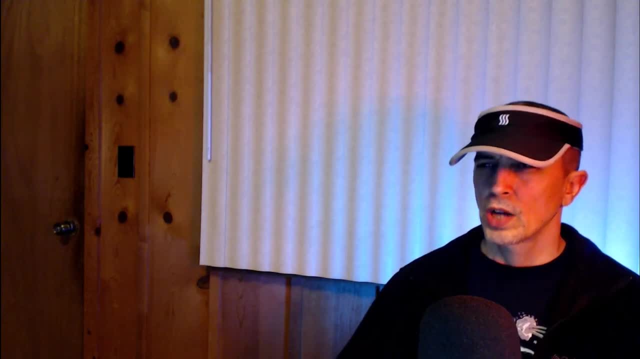 the programming world, just like JavaScript is the one of the most benevolent and loved entities, even as it passes, as it changes hands, because JavaScript has changed hands of ownership over the years. I think it's Oracle now that owns JavaScript. I'm not exactly sure, but it changes hands. so 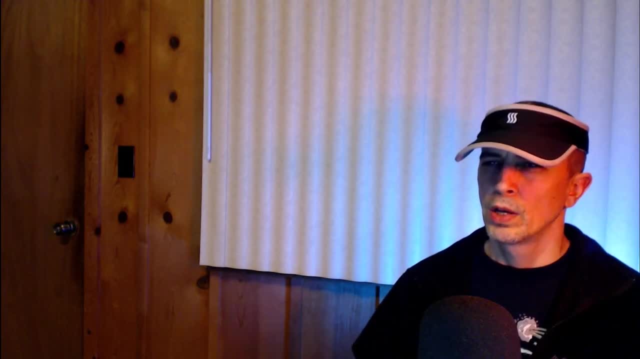 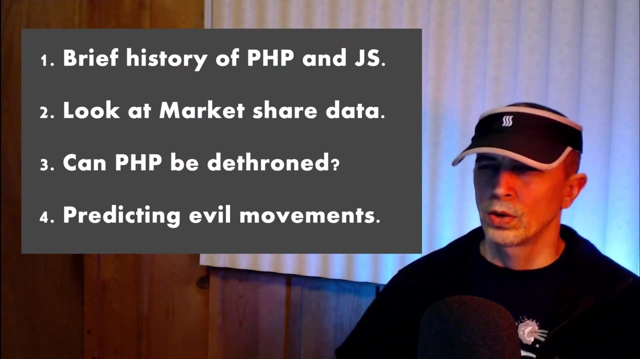 many times of who's managing it and has ownership over the brand of JavaScript. now I'm going to add one more item to the topics on this video, which is where and why I get critical of other developers. when I get critical, maybe judgmental, and you remember I made the video of framework snafus and pitfalls. 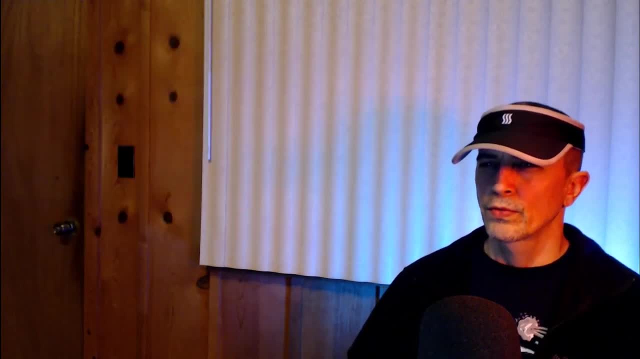 where I prove all of the downsides of using frameworks and how they're not actually productive but counterproductive to a developer's long-term life or long-term career, and before I jump into that topic of why I get critical of others and their development practices I wanted to discuss, remember, in the beginning of 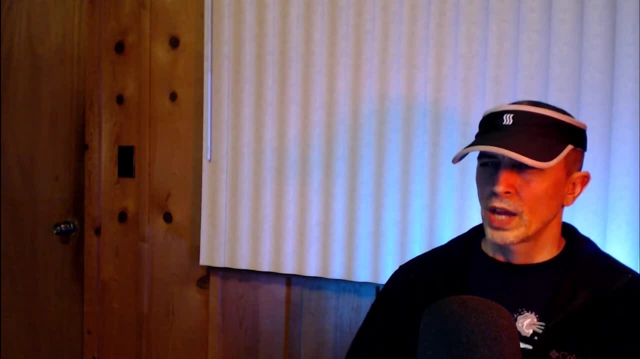 the video I said that the majority of humans can be wrong, and the fact that the majority of humans believe or think a certain way doesn't mean they're right about that just because it's the majority. the best example of this is in the spiritual philosophies of the spiritual philosophies of the spiritual. 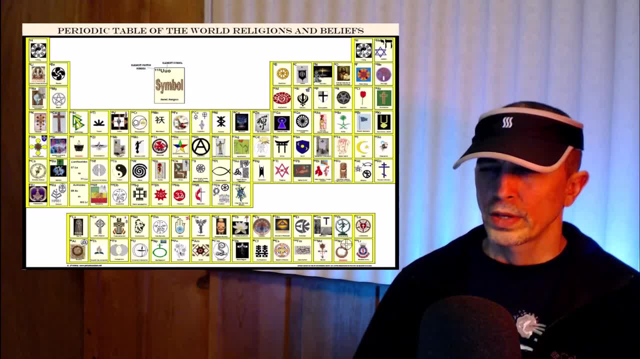 and religions arena. now first, before I get into this, you should know that I'm not an atheist and I'm more of an agnostic that claims to know nothing in an absolute sense. I don't claim to know what is going on in the spiritual realm. I 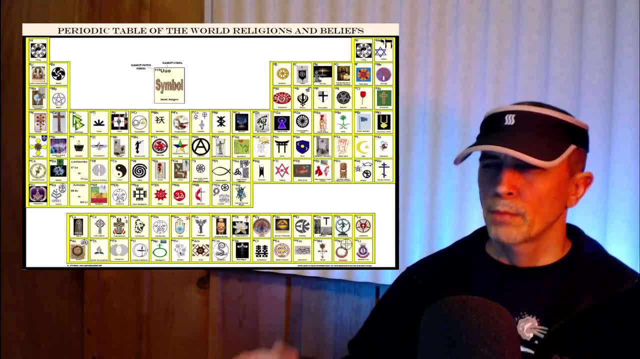 do have my own notions, kind of like my own spiritual philosophy, and I do believe I have a weird belief or a unique belief, which I'm not alone in this, but it's kind of rare. I believe that existence and all of creation is sung or brought into being by 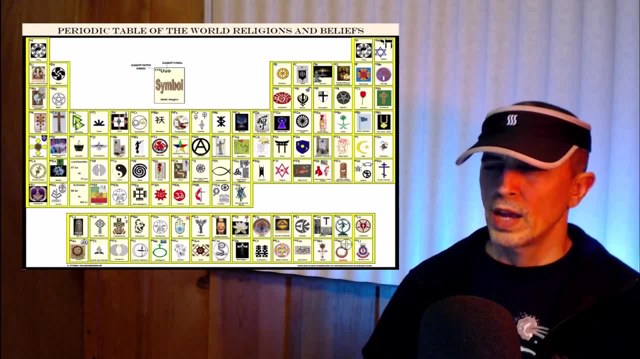 sound and vibrations. I believe the Creator has sung the universe into existence, not by actual song that you can hear, but I'm talking about sound frequency and vibration, and you can see this if you study cymatics. I don't know if many of you know about cymatics. 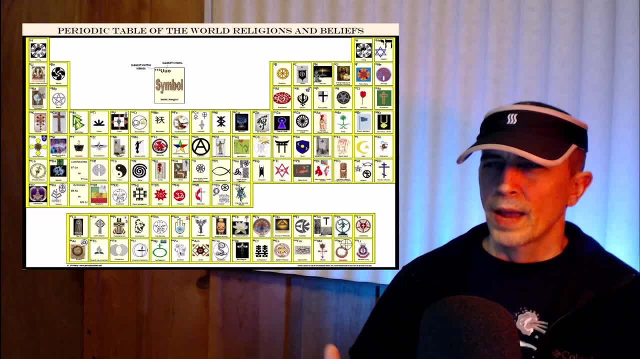 some of you probably do, but you can see cymatics playing out at the macro level and the micro level, for instance at the, the poles of the large gas giant planets like Saturn and Jupiter. you can see geometrical patterns being formed by the vibration, sound and frequencies coming off the planet themselves, and they've 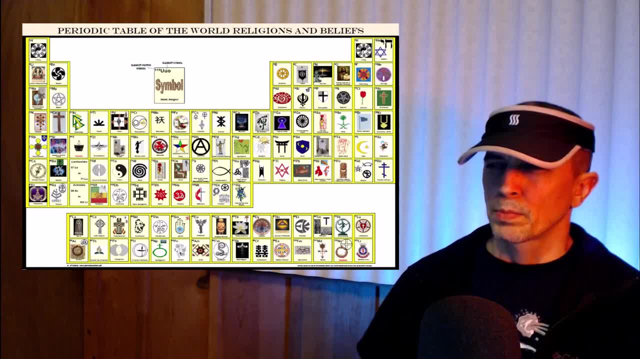 put audio instruments, these planets and the sounds they make and you can hear definite cymatics and that's how you get this hexagonal geometric pattern on the poles of, especially, Jupiter. it's really evident. so that's what I believe. I believe that sound and frequency is what creates the material universe and keeps 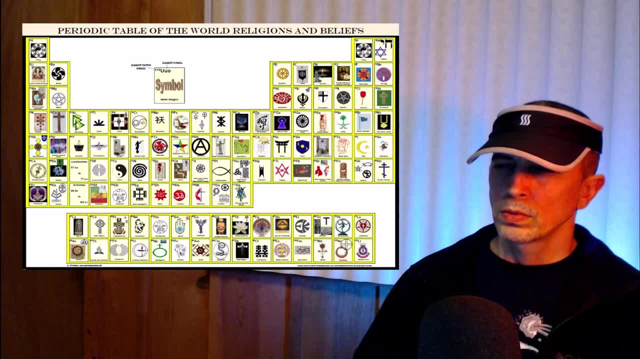 everything with a structure at the atomic level, the micro level and at the macro level. so I don't believe that everything is just chance. I think that something has sung all of this into existence and there's a lot of ancient philosophies that believe that the great spirit or the most high 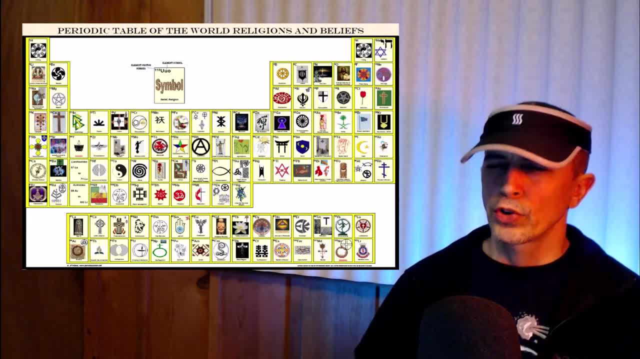 has spoken word from that being that entities has created all that we see and know. and even in the abrahamic religions, god, spoken word, created the earth and the heavens. so that's what i believe, but i don't believe it absolutely. it's just some feeling that i have in my gut. so now let's get into how most humans can be wrong. so we have. 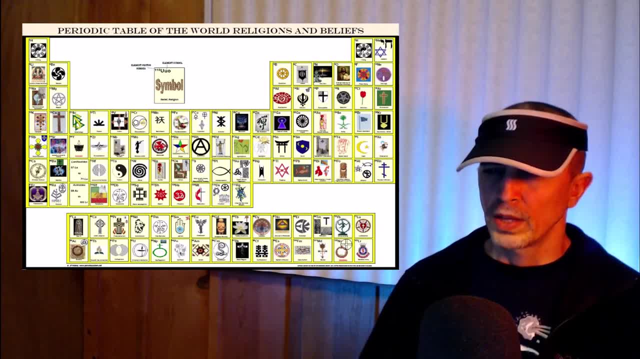 developed over 5 000 different religions and spiritual philosophies over recorded history, which are actually just frameworks that we use for morality and for attempting to describe what we all observe and feel, whether you be a hindu, yogi or a buddhist master, a jewish rabbi, a muslim. 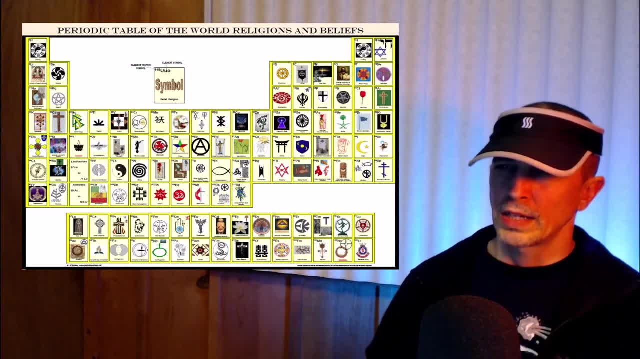 imam, or even the pope of christianity or some kind of cardinal. these are all just different spiritual frameworks that we use. now we can't all be right. all of these religions that we use are just frameworks that we use and we can't all be right all of. 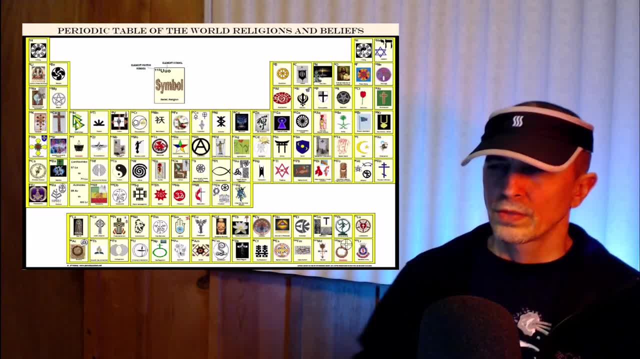 these religions that we use are just frameworks that we use and we can't all be right. all of these 5,000 different religions and all the thousands of gods that revolve around these religions. it can't all be right and true. So that means, by logic alone, most humans are wrong. 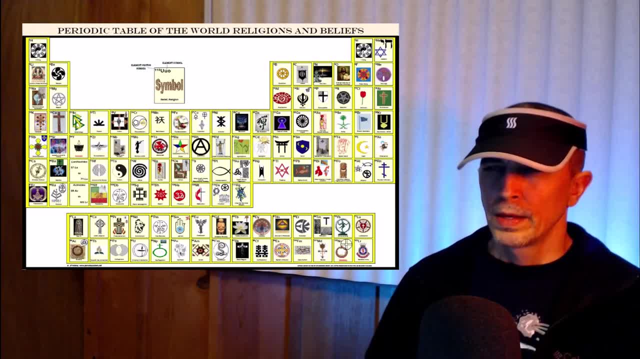 about their spiritual notions, And even my spiritual notion could be just dead wrong and I'm not going to stand and die on that hill, But religion and spiritual philosophies prove that most humans are wrong, And it doesn't mean that just because the majority of people. 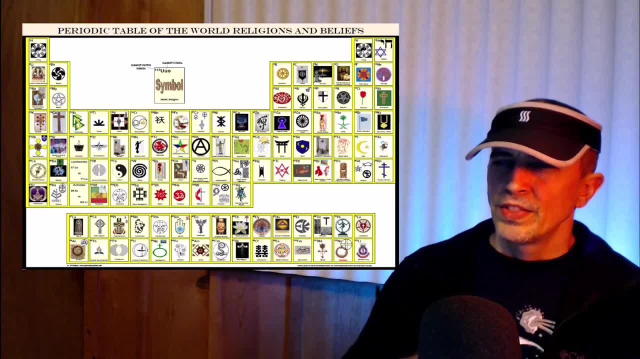 are religious means that that is true, Because it could be that God or the Creator is behind just one specific religion, which would be the only one true religion, and that would still make so even if God is behind one true religion, which is probably not the case, but even 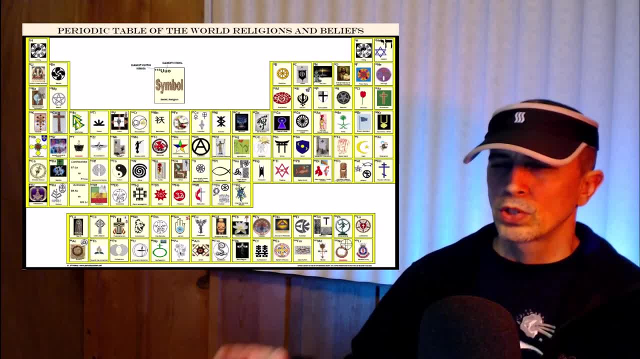 even if that is the case, that means most humans in the world are wrong and going down the wrong path And only the people in that one true religion, which would be a minority and not the majority, those would be people on the right path. But I don't believe that's the case. I believe that 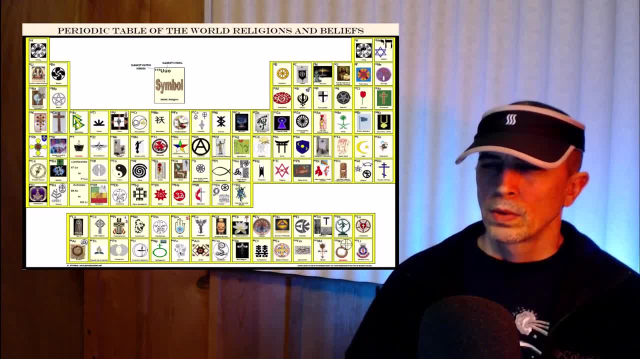 we're all equally wrong at some degree in our attempts to explain creation and in all of our spiritual philosophies. I believe we're all more wrong than we are right. So that's one example of where the majority of humans could have notions that are not actually true. but just because the 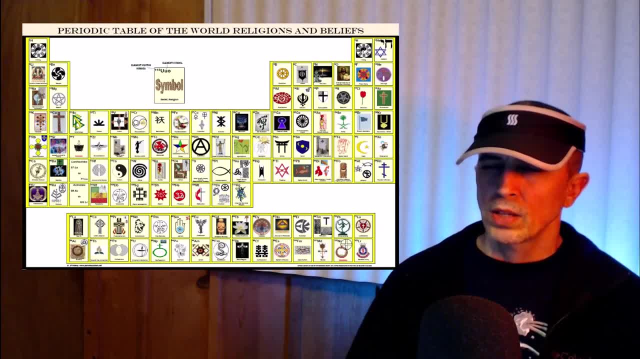 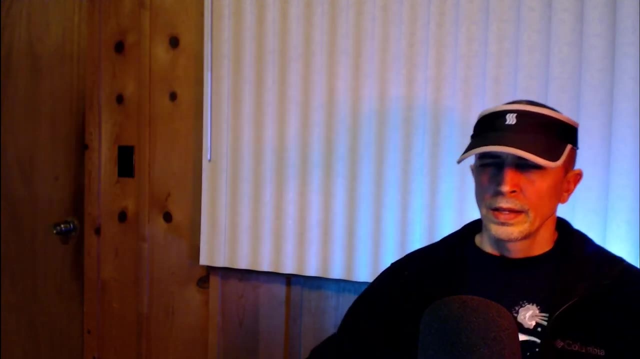 majority of people believe it to be true, it doesn't make it right and it doesn't make it the truth. So I just wanted to compare that to the development world where, just because the majority of developers believe a certain thing, it doesn't make it true. They could all be misguided and wrong. 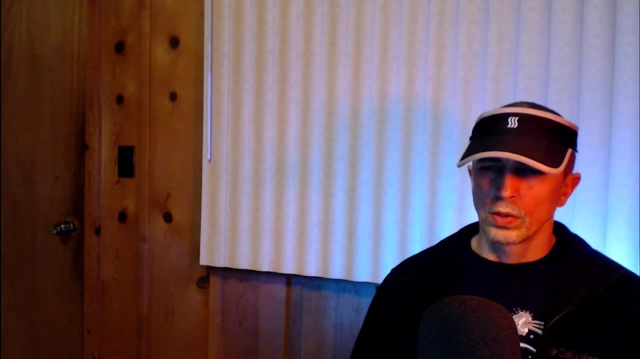 Now, finally, I want to quickly discuss where I get critical and disappointed in modern developers. And it happens when developers disregard the raw beauty and the ease of use of both PHP and JavaScript, And this is why we have an oversaturation of frameworks. 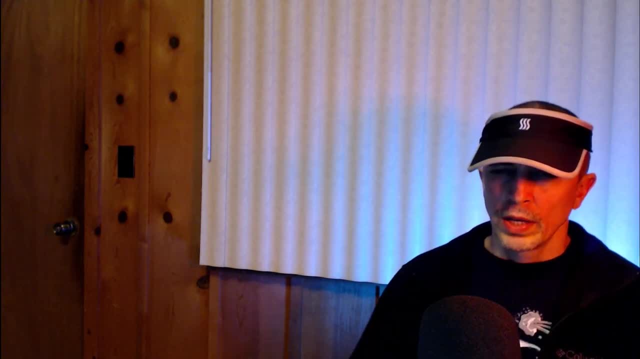 I think that these developers are types that are brainwashed, new green developers, and weak, lazy minded developers that perpetuate a set of lies, because these lies help them feel equal to seasoned and strong developers, which they are not. Not all humans are created equal, And that's why we have 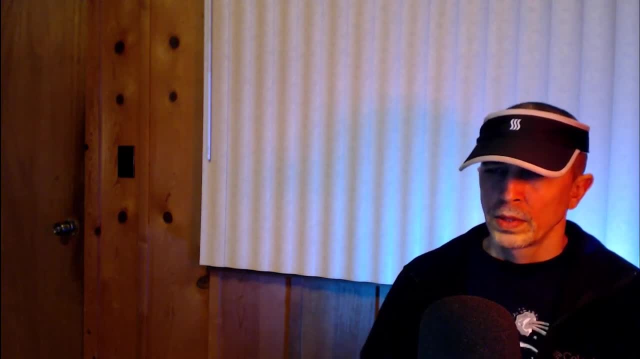 the mess that we have today. These simple, free languages were never intended to be abstracted all to hell, in a general sense, by what is now thousands of frameworks that exist only to make their specific authors rich or popular, Because what happened is people saw things like jQuery or Cake. PHP become really popular and the developers of those frameworks got really popular, wealthy and famous. So everybody's trying to go down that road and become the next, Whatever, For financial reasons And for greed. basically, They're muddying the waters of these. 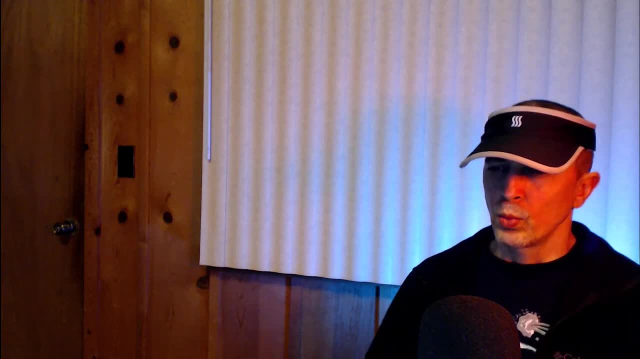 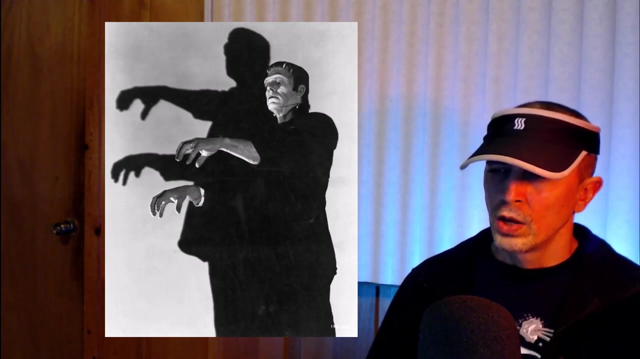 beautiful languages like PHP and JavaScript. Now weak, lazy minded developers. they use a set of excuses for why they use these frameworks and why they develop heavily bloated, slower loading Frankenstein projects. These excuses worked when only jQuery or Cake PHP had dominance. Which was years ago, There was only jQuery And there was only Cake, PHP and a few other frameworks And they had dominance over the whole arena, But not complete dominance, because more people were still core JavaScript focused And not jQuery focused, For instance, people like me. I knew that jQuery was not. 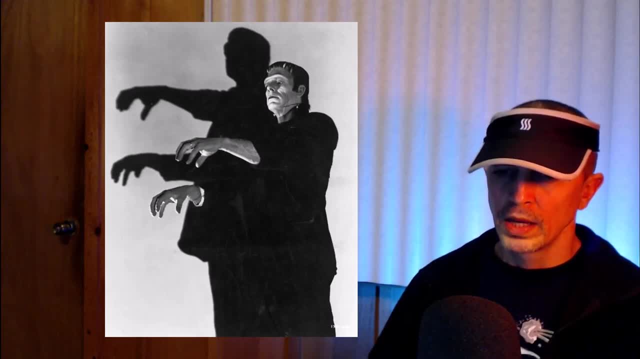 going to last forever. so I didn't invest much of my time in learning its code base And I knew that its code with simply an abstraction layer above the already easy to use JavaScript core language. So now what we have are many thousands of frameworks with low conformity among their. 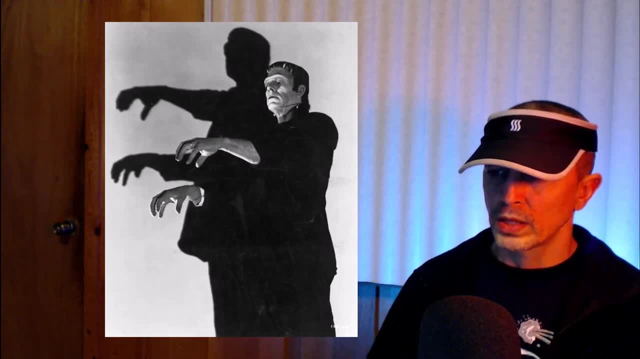 code bases. So the excuses used by weak developers or ignorant business owners, they don't stand up well now. These excuses do not stand up well now. For instance, the main excuse used, which is it's easier to bring in new developers into the project. That excuse does not. 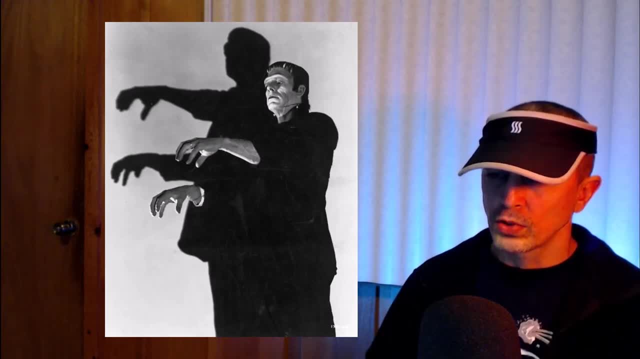 stand up well now because there are thousands of different frameworks, each with a different code base. So a modern developer knowing just one or two frameworks code base really well would only be useful to a very small handful of clients or businesses, Not even close to being useful to all. 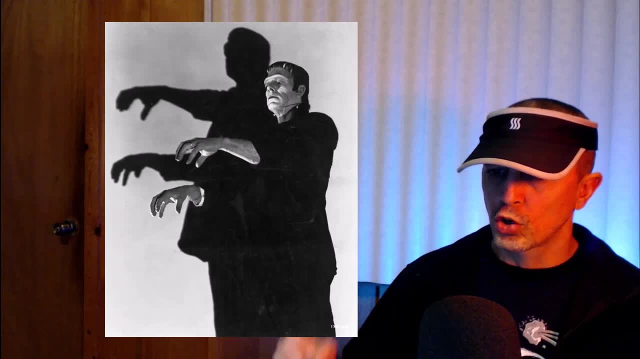 of them. So the main excuse used, which is it's easier to bring in new developers into the project, That excuse does not stand up well now, because there are thousands of different frameworks, each of them Now, on the flip side of that, knowing just the core language really well, for instance, JavaScript or PHP, if you know the core language really well- would bring a higher level of production speed and a much higher level of code base conformity to all projects worldwide. For instance, a Vue or React developer will not be any more useful to a jQuery. 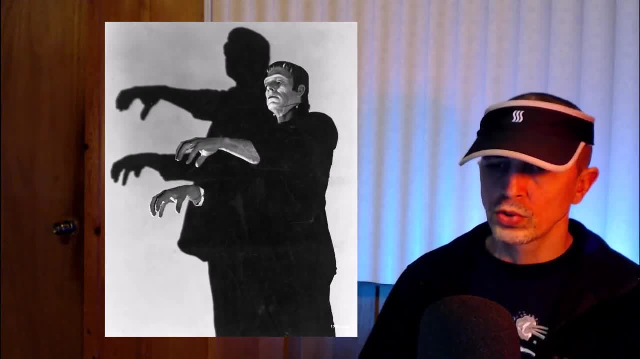 or node driven company. They won't be any more useful than some person who knows the core language extremely well, And I believe it's the opposite: The person who knows the core language extremely well will be way more useful in this myriad of frameworks to. where they don't have to go learning all of these thousands of frameworks. If they just focus on the core language, they'll be a much faster, speedier developer in any company that requires JavaScript or PHP code on whatever abstraction layer that it may be written on. 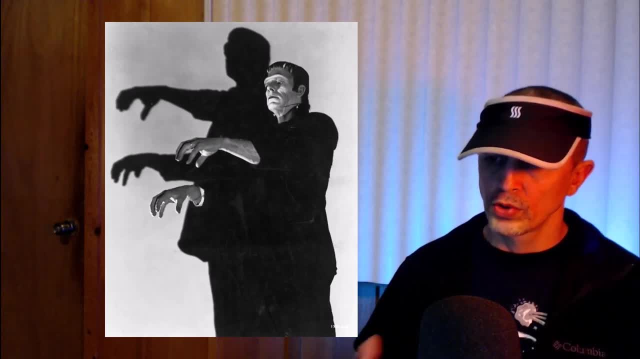 So the core language focused developer is now more useful to all companies in a broader sense, due to having a higher level of knowledge about how things really work under the hood People who get caught up in these frameworks- they don't even understand how things work under. 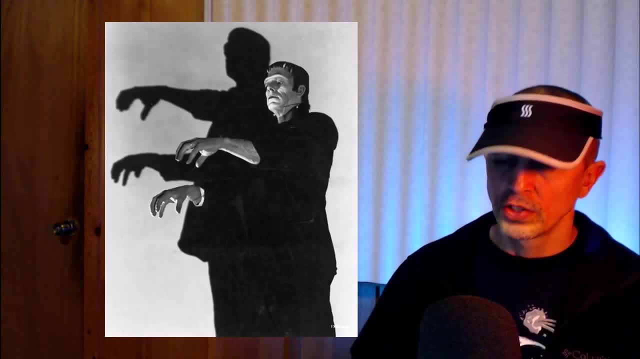 the hood. When the core focused developer does really well, they understand what's happening under the hood of these machines. Another excuse that people want to find when trying to figure out how to handle a topic that is really difficult and that isn't use is that the code is more secure, and this is also a lie, and I proved how this is untrue. 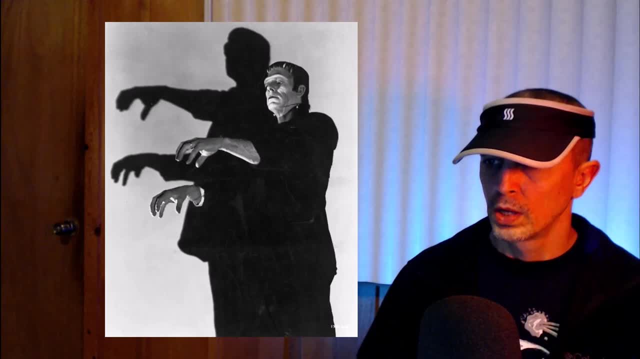 in my framework pitfalls and snafus video which you can watch here later, and I'll put a link to that video right now on top of this video, on top on the top right, so you can click on it if you want to watch it now. but you can also wait till the end and I'll put a 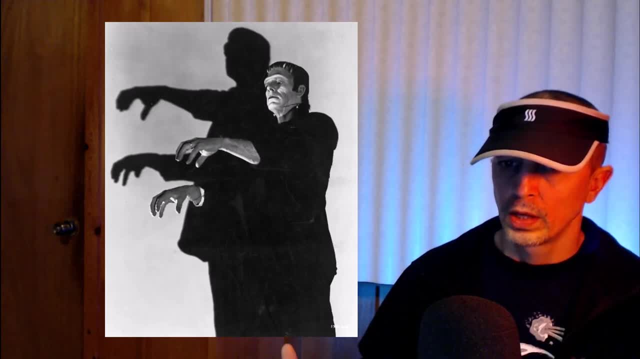 link to that video on the end screen, on a card. that way, at the very end of this video, you can watch my framework, pitfalls and snafus video, which exposes a whole lot of the mess, and in that video I explain what kinds of frameworks and libraries are productive to. 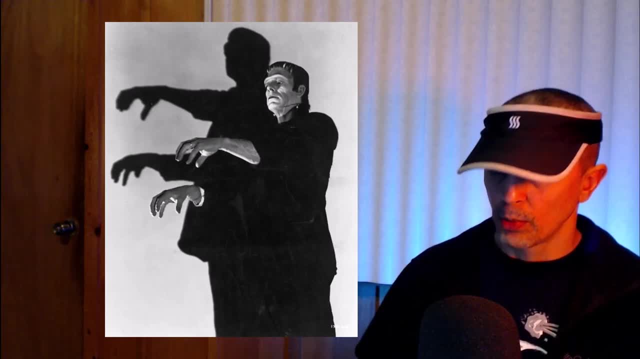 a developer's career, because not all of these frameworks- most of these frameworks- are counterproductive to a developer's long-term career, but a few of these frameworks are really productive to a developer's short-term goals, and I explained which one those are and I also explained in that video how a team or a single developer even can create in-house. 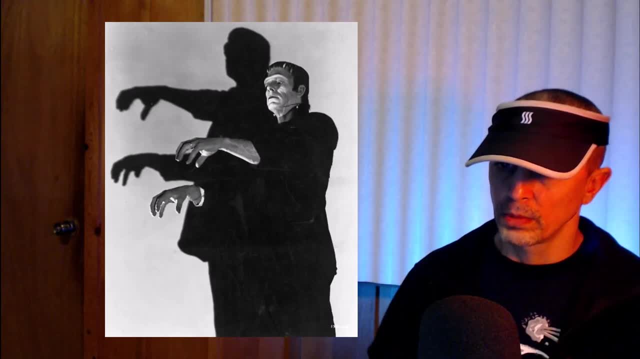 class files for ease of use for new team members that they bring in, or if they have to be replaced themselves. the next guy can easily pick up. if he knows programming well, he can easily pick up where that guy left off if the class files are all in place. so javascript and php. 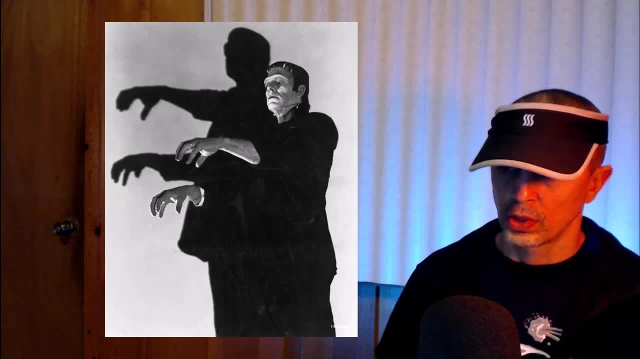 are not difficult enough to use to warrant the existence of what is now thousands of frameworks that have confused the languages and have muddied the waters of what is two beautiful, easy-to-use technologies that should be. developers should be focusing on the core of those languages. 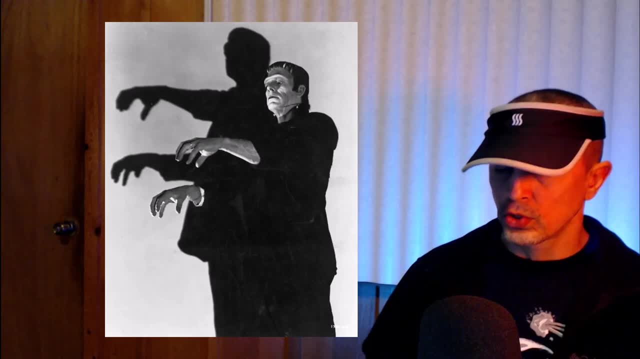 instead of these thousands of frameworks. so in the future, if we keep down this path of confusion and muddying the waters and greed dominating the market, there will be no code-based conformance or easy sharing of code between the global community and the market. so the people who are 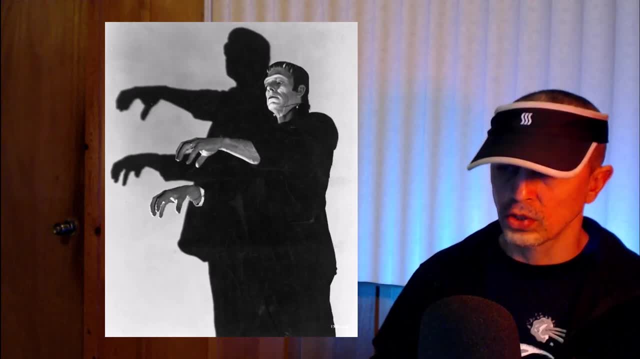 developers. if we keep down this nonsensical road of abstracting php and javascript, all to hell and back, and the same logic applies to all core programming languages that frameworks are developed for. we have become like the confused language tribes after god punished man for attempting to build the rickety tower of babel. now i'm not religious, but that story reminds me. 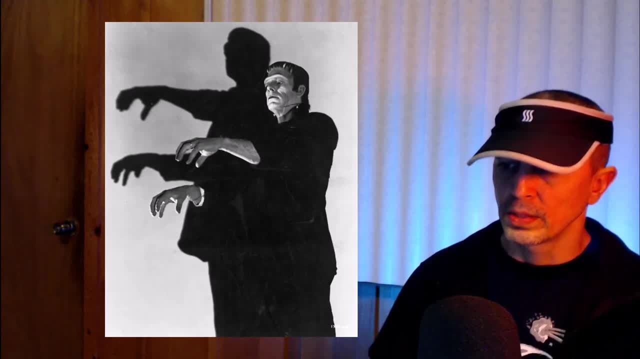 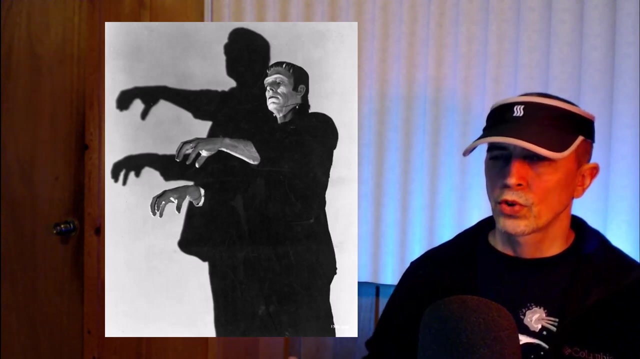 of what we have done regarding frameworks in the programming world. we're confusing and oversaturating what is already an elegant and common sense way to be. we are self-destructing the programming world basically now. i think that's basically all i have to say. and php is king of server-side programming for the web, javascript in its 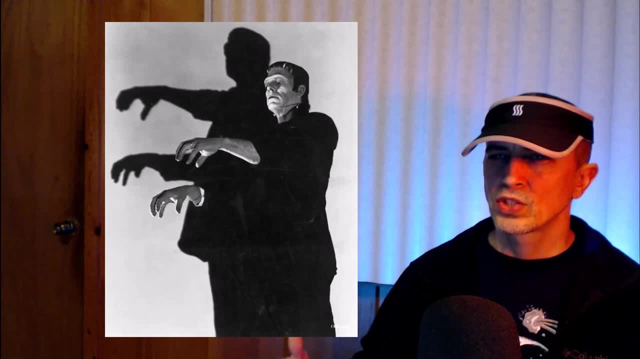 unobstructed raw core programming world is king of client-side front-end development, and that's the reality. all of these frameworks are going to come and go. they only have a short life usually. just look at jquery. jquery used to be the dominant thing just a few years ago and now it's falling out of grace. but javascript. 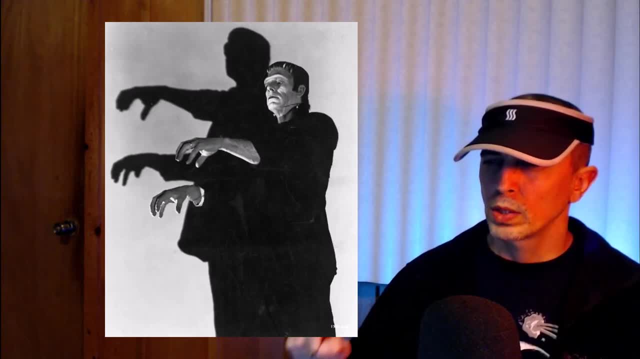 will last. javascript at its core will last. so i urge developers to concentrate on the core of javascript and focus more on what they use to do, understating that framework, than you do all of these frameworks, and if you do that, you'll be more easily able to. 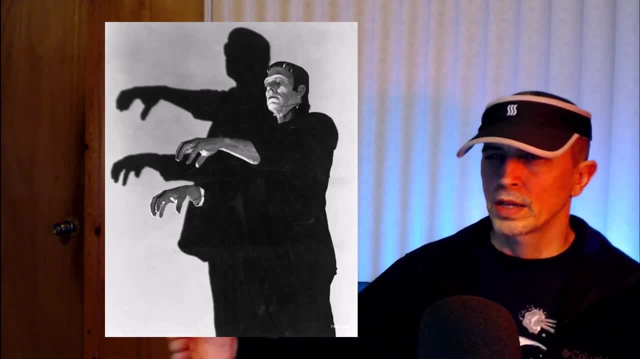 bounce between client 1 and client 2 or company 1 and company 2, no matter what framework those companies are using, because if you understand the core of these languages, you'll be able to bounce around all of these thousands of frameworks more easily and you won't have 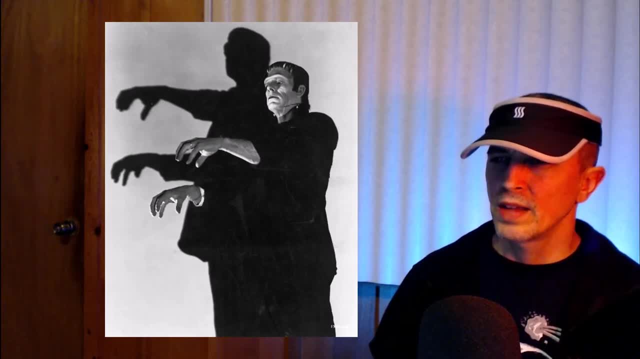 to learn all of these thousands of frameworks, typically because they only have a large value of frameworks, so in depth, for instance, I could jump right into node, I can jump right into react, I could jump right into view and use all of them relatively quickly and easily without having to invest my career in that framework and 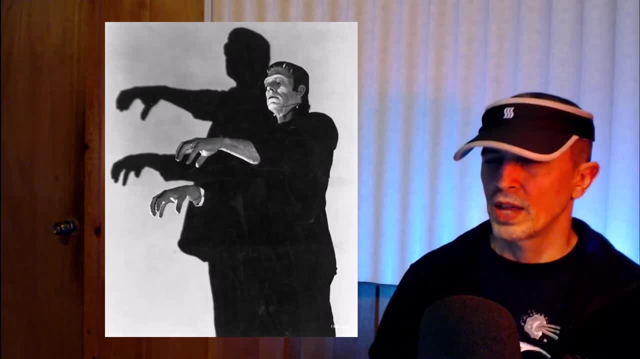 I'll be way more useful and handy to companies that can't use those frameworks. what if you get hired by a company that wants to create a framework? you can't build a framework on top of a framework and, unless you run a big rickety system, if you want to create a new framework, that's going to get popular. 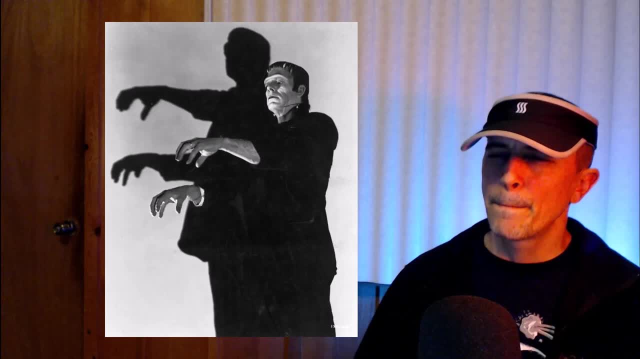 and that you're gonna get rich off of. it has to be built using JavaScript core, and then you try to get it popular and have thousands of people start using it, and then how? that's how you launch your, but it can't be built on the back of.